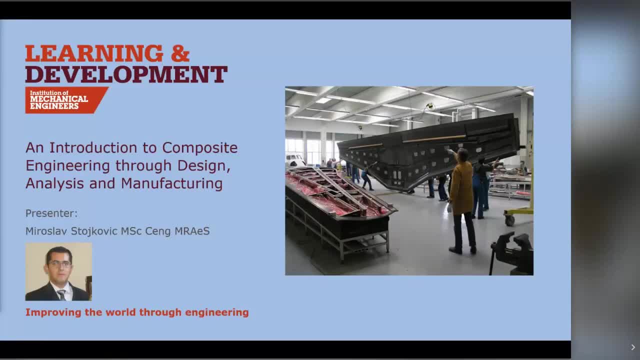 to the presenter in readiness for the for the Q&A time at the end. Okay, so without further ado, I'm now going to hand you over to today's presenter, Miroslav Stozovic, and I'll hand you over. okay, over to you, Miroslav. 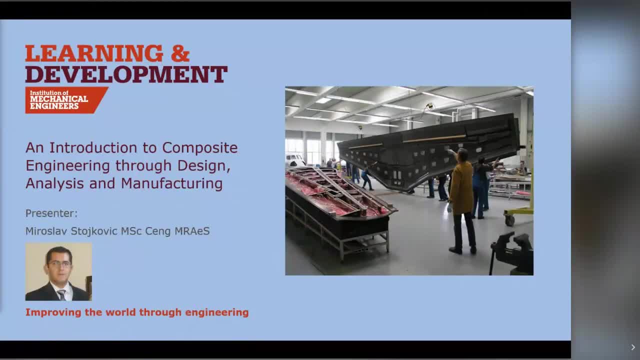 Good afternoon everybody. my name is Miroslav and I'm your presenter for today. I will tell you a little bit about my background and then carry on talking about an interesting topic of composites. So I've spent my years in a variety of 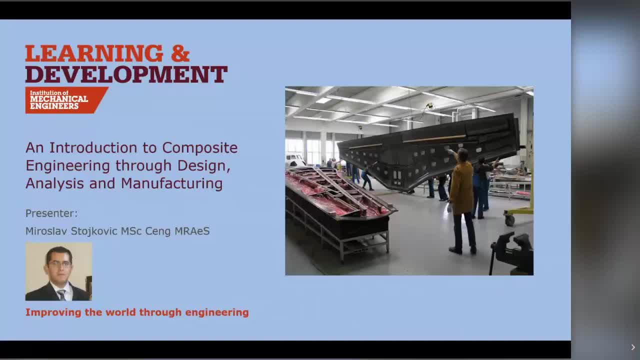 regulated industries and catering also for research and development and also looking into composite development, lifecycle manufacturing and research and R&D. So hopefully I'll be able to give you a bit of a background of why composites are so interesting, important and useful in a variety of engineering applications. 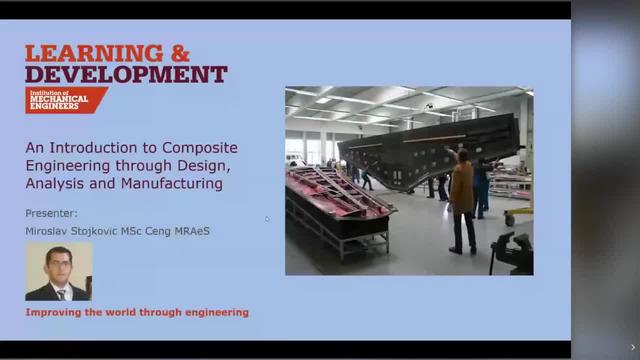 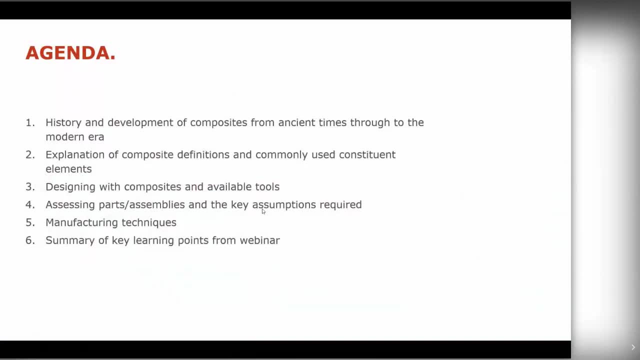 So, without further ado, I will introduce the today's presentation. We'll start from looking at the history of composites and where the origins of composite materials and thought of composite materials come from. I will explain some basic definitions that are commonly used across engineering and manufacturing. 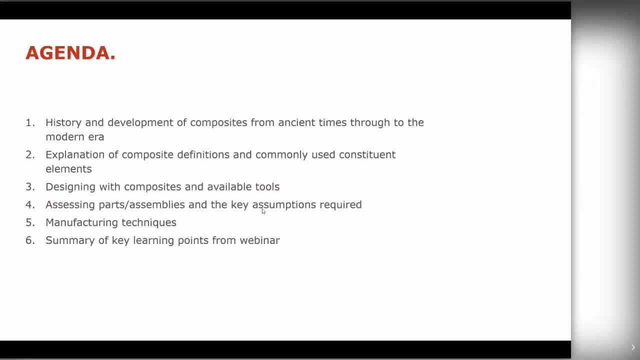 in the composite world. We'll touch upon designing or how to design with composites, once we have learned some of the definitions and what composites are, And we'll be talking about how to manage parts, assemblies and some key assumptions built into into this. And, very, very importantly, we'll be talking about manufacturing techniques, because 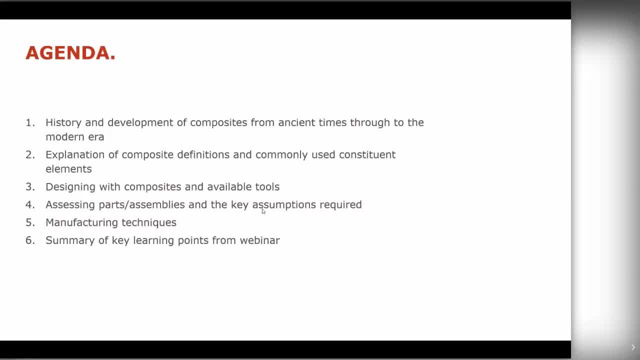 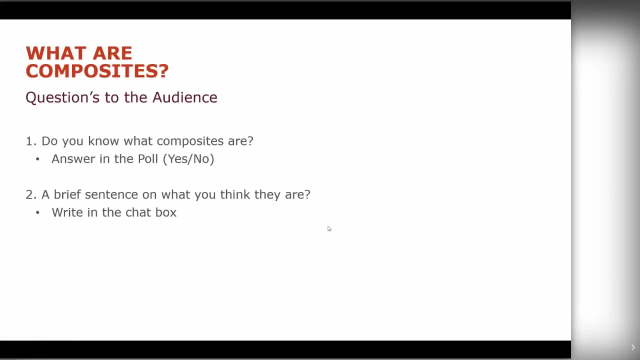 composites are so different to other manufacturing processes that manufacturing plays such a significant role and is inseparable from design development process. and we finally end with summarizing the key learnings and what have actually been through today in this webinar. So, before we actually start going through the presentation, I would like to ask a couple of questions and you can answer to the poll. 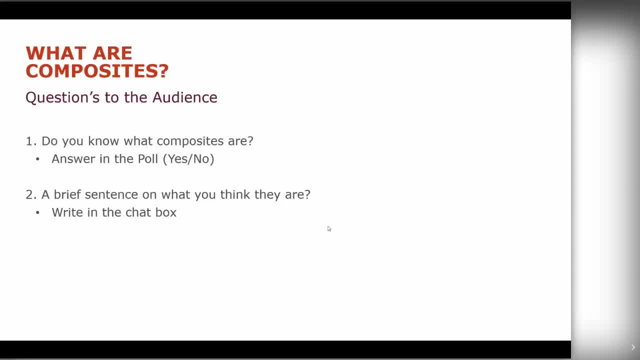 First one is: do you know what composites are? And it's a very simple yes, no type answer. And if you do know what composites are, could you please write a little description in the chat box And we'll later on reveal some of the possible possibilities of what composites definitions are. 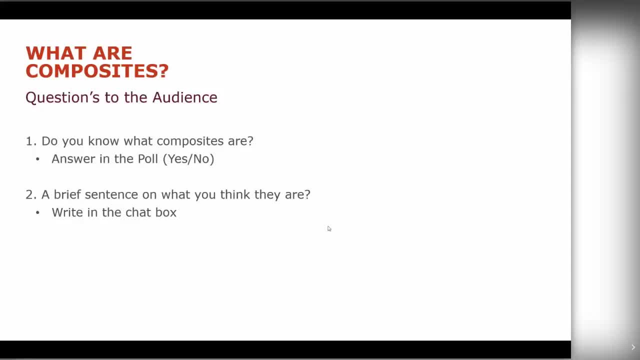 So we'll give you some time to do so. Are we ready to publish the results, Miroslav? can you see the results there? No, I can't actually. I'll just say, out of the yes and no's, 88 percent are yes and 11 percent are no. 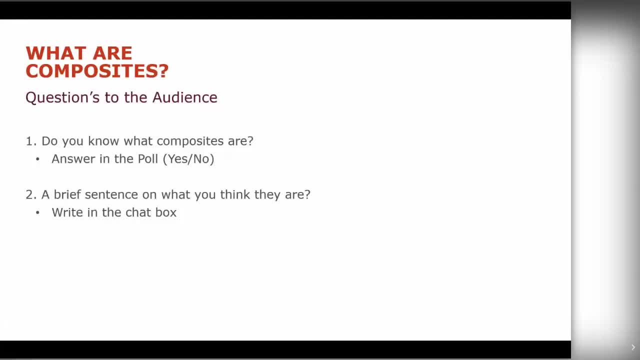 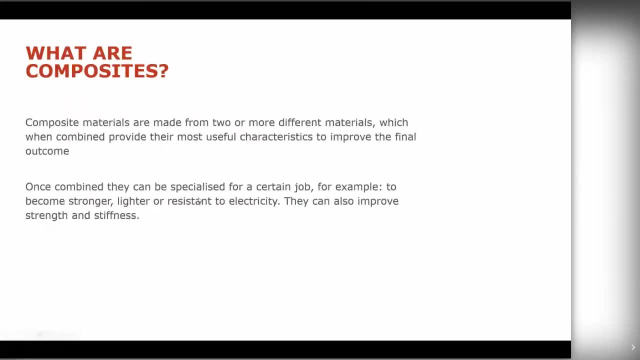 OK, that's, that's fine, So, Effectively. composites are materials that are formed by adding to existing materials to exploit their mutual benefits, And the implication is that the composite material can use the properties of whatever the constituent materials are built. 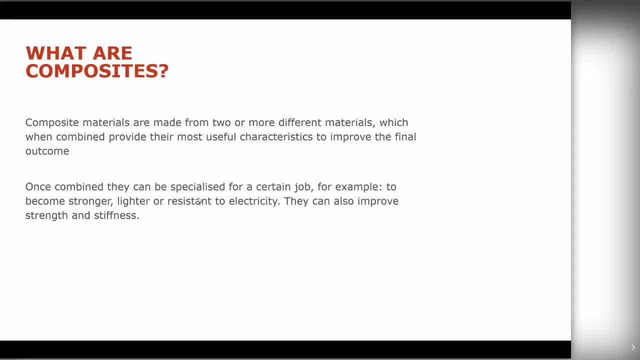 built into. So the final product is actually much more improved material than the two constituents to start with. What this also means is that we can tailor the composite to have the properties of the constituent materials to cater for strength, stiffness, But also we could add materials that are resistant to electricity or, if need be, 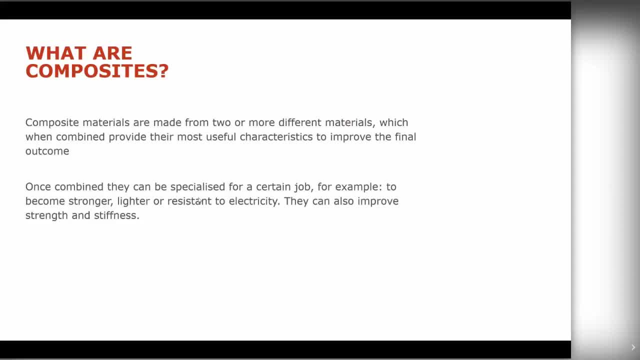 add material that is either electrically conductive or electromagnetically conductive. So there is a variety of uses of how composite materials could be, could be functionalized, But the key important message is that the composites are a combination of two or more constituent materials to exploit the mutual benefits. for whatever the design, final design goal is. 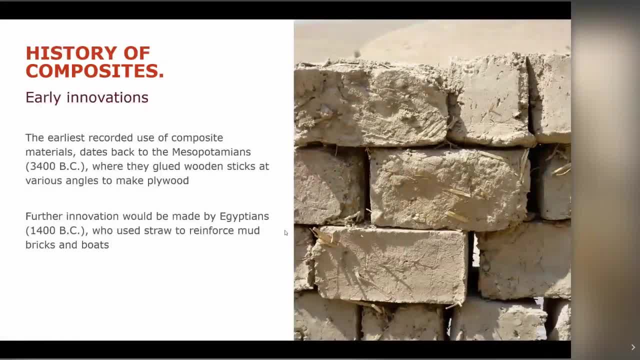 So I said we're going to start by reviewing a history of composites, And in this slide you can see that we started very, very early. Human thought has used materials such as wooden sticks and mud to create bricks, And you can see some some historical information. 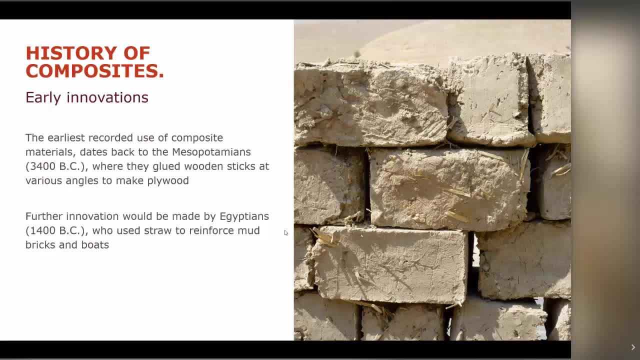 But the key thing is, humans have tried to reinforce basic mud material with straws, which is effectively what composites do. Fiber in the modern composite material are actually doing exactly the same function as the straw sticks in this, in these mud bricks, They're reinforcing material in particular direction, giving it strength and stiffness. 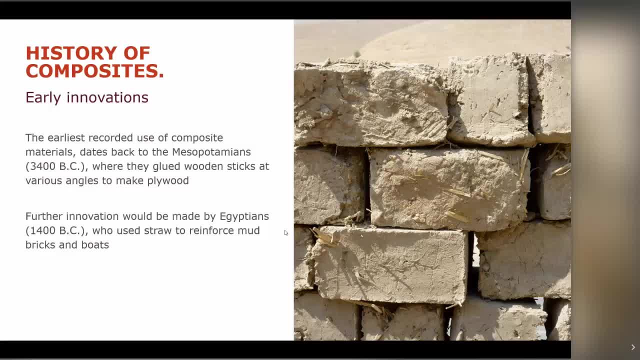 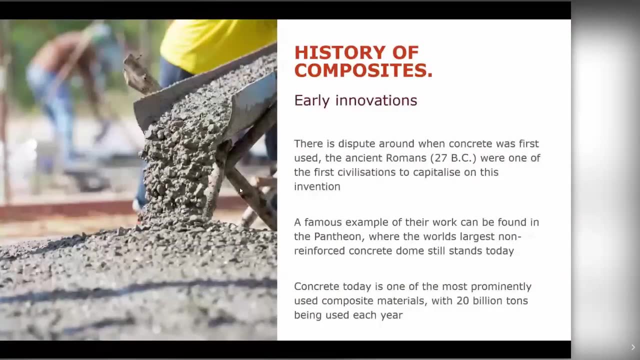 And you can see some examples from more than 3000 years ago of these ideas being tried to use by by by humans. Some other examples, or rather very early examples of composites, Include a concrete. concrete in itself is a composite material because it is a combination of number of of different constituents. 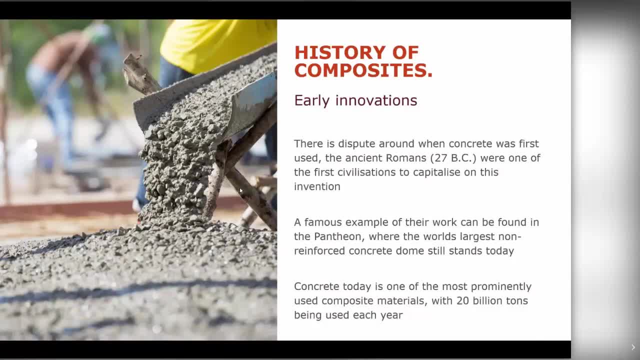 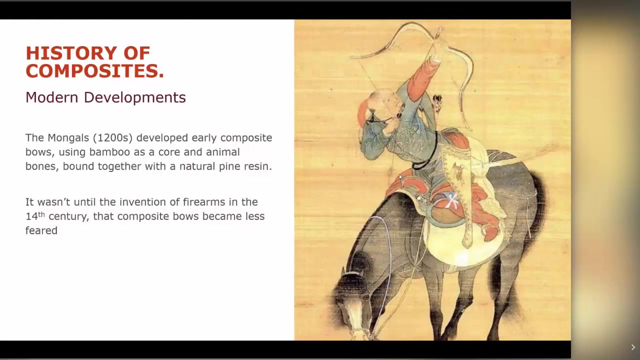 If you then reinforce it, that further strengthen up the composite material. So the steel reinforcement acts as additional material and therefore it is also classed as a composite material. Moving on from from these developments, you can see that there were some, also early, examples of using composite materials in developing weapons. 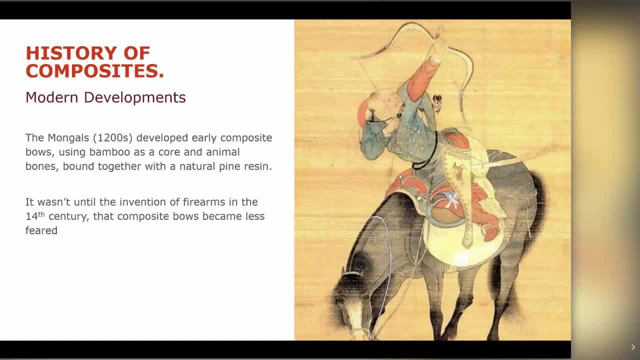 So Mongols have used the what is early composite by combining bamboo and core animal bones together, bound with the resin, to create material which was light, stiff and gave them properties needed for construction, needed for for bows to effectively hunt or fight. but this is all quite old and these are the 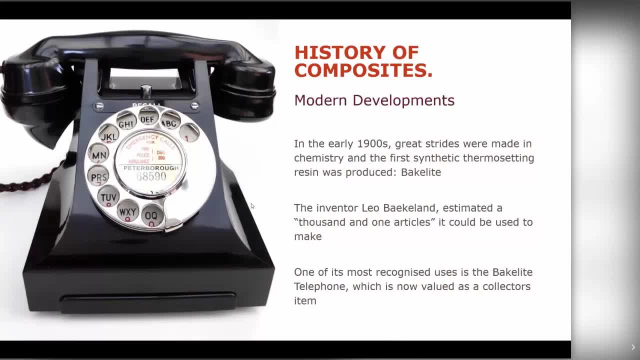 materials that humans could find in nature. effectively, what actually turned around the history of composites was introduction of plastics as a reinforcement material. so one of the key turning points in history was introduction of baklite, which was used, for example, for old-fashioned phones like one presented in this picture. 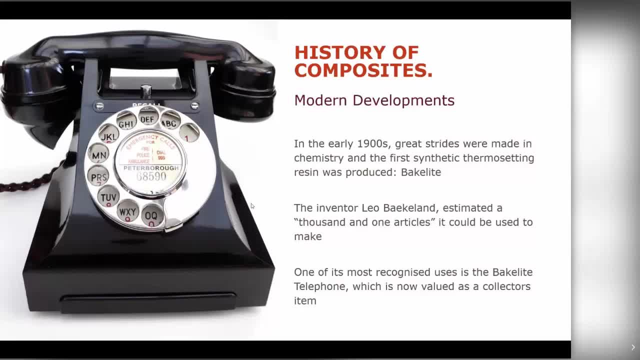 and that is effectively thermosetting resin. that is, and thermosetting resins are one of the constituents that make the composites you'll see a little bit later. so this was one of the turning points: introduction of engineering plastics that made it possible to produce plastics with. 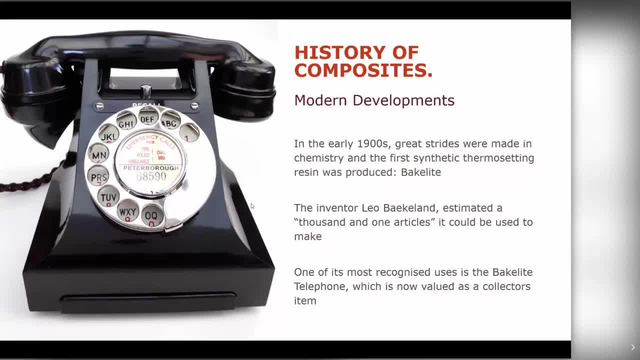 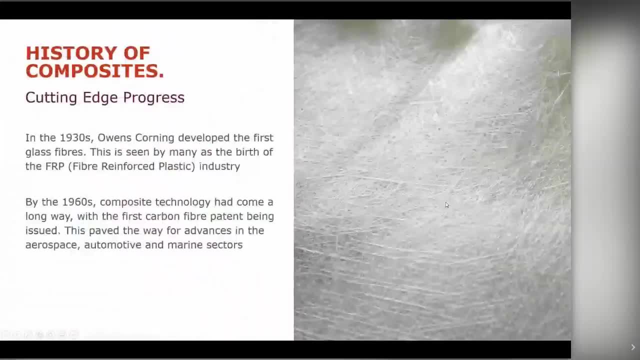 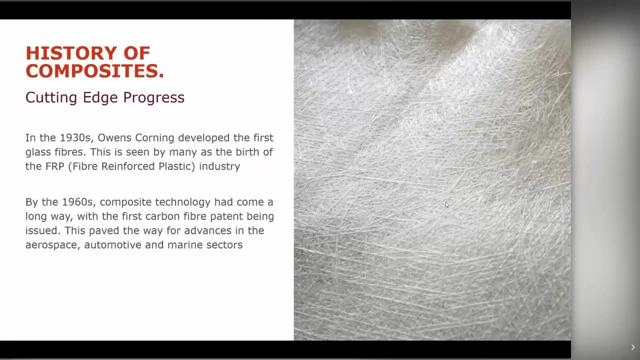 known properties, homogeneous materials and standardized manufacturing processes. the other component that made it possible to actually make composites into engineering materials, like we know today, is introduction of fiber. so in 1930s owens corning developed first class fibers and this is again seen as another turning point in the 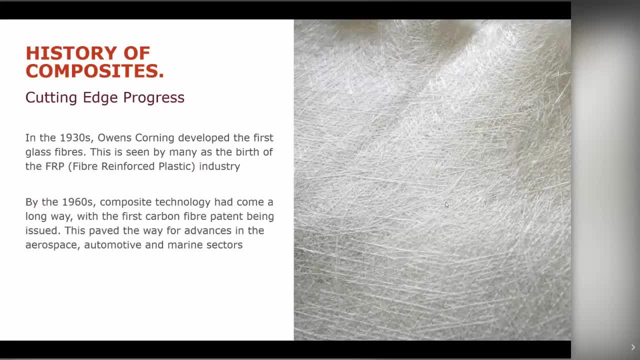 development of fiber reinforced plastics industry. so by introduction of resins or thermosetting resins as a matrix material and fiber or engineering manufacturing- a commercial way of making fiber- into the market made it possible to make composites or start to make composites in a way that is known to us today. 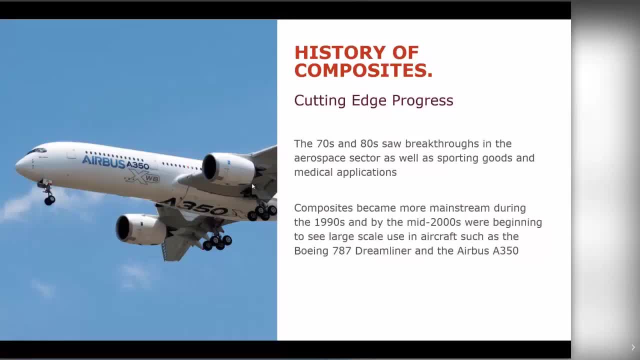 so since then composites took off and in 70s and 80s composites were started to be used more and more in aerospace sector, although i do have to say there are examples, very early examples, of aerospace sector using composites much earlier than 70s and 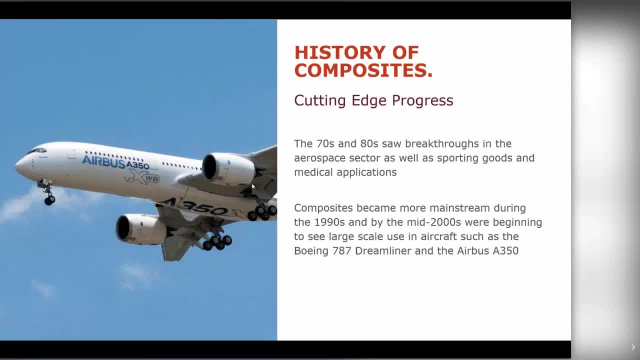 80s. however, it was only in the 90s and 2000s when the large commercial use of composites in aerospace took place by introduction introducing composites into design and development of a large aeroplane such as 787 a350. so that's kind of a very short history of 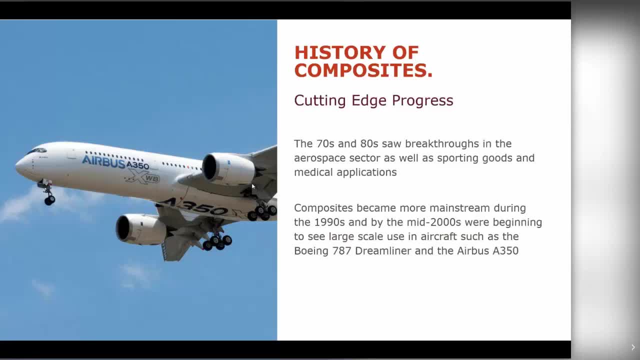 composite thought, starting from very early ideas of reinforcing some material by having some strong and stiff fibers in particular directions, and that thought carried through the history of humankind and it was few turning points that made it possible to have the, that reinforcement material, produced in a standardized manufacturing fashion and 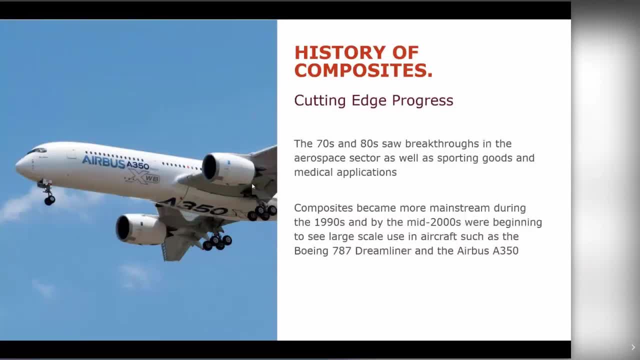 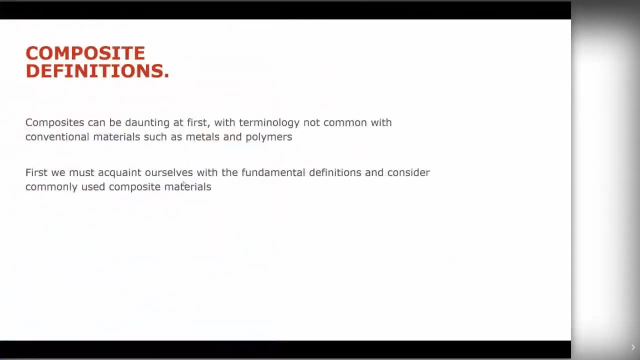 also the resin to be produced in a standard manufacturing fashion made it possible to use composites in a way that we do now in examples such as this aeroplane here in the picture. so after this very brief, short introduction of history of composites, i'll introduce some composite. 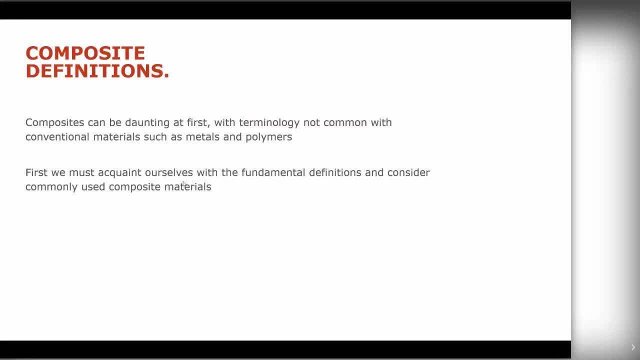 uh definitions. there is loads of uh definitions and terms within the composite uh- material science, manufacturing and design- and it's very important we know some of those so we can actually have the construction, constructive discussion and the carry out design and manufacturing. so let's start with the um. 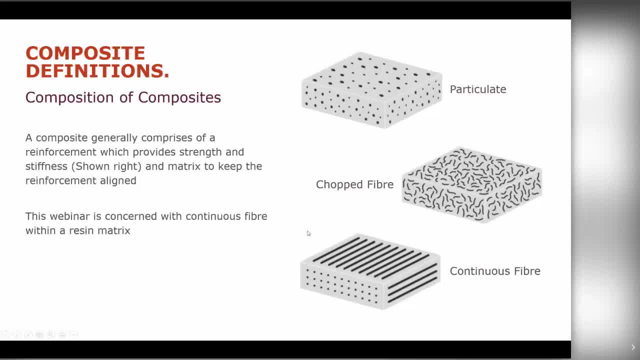 what composites are. so i mentioned before, from this historical overview, that uh composite is generally comprised of uh, uh, reinforcements, uh, which provides strength and stiffness, and in in the case of these three pictures, you can see some continuous fiber, chopped fiber or particulates, which are effectively. 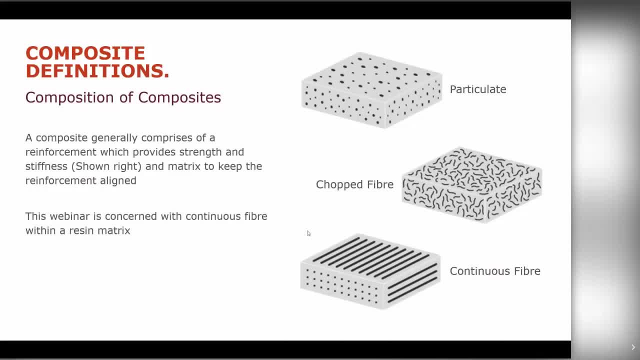 providing this uh, strength and stiffness, and the matrix, which is also known as uh, as resin uh, that keeps those fiber together. you can see that the uh composites uh or resin matrices uh, and also on continuous fiber. so uh, uh, uh. what we are typically using in engineering practice for some high value articles are 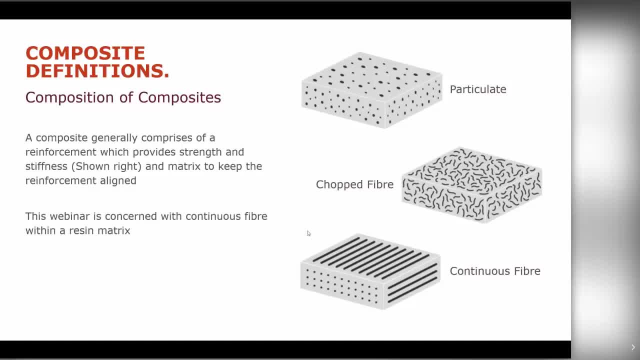 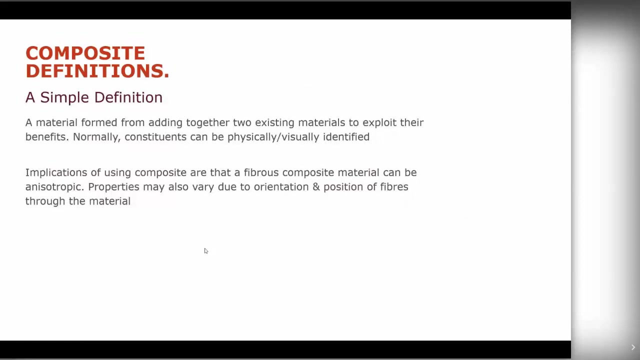 continuous fibre composites and also the organics matrix materials, resin matrices combined into composite material. So this particular webinar is concerned with this type of material. I said before that the composites are materials that are formed by adding together two existing materials to actually superimpose their properties and create a material whose properties 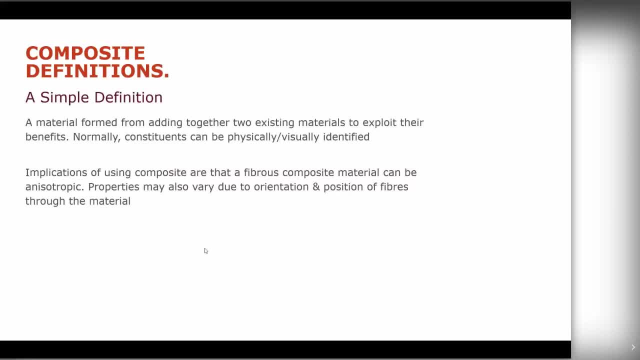 are better than the properties of those two materials separately, and that's really the definition of what composites are. Another layer on the top of that is those constituencies could be physically or visually identified. So they're not mixed as chemical mixtures. they're. 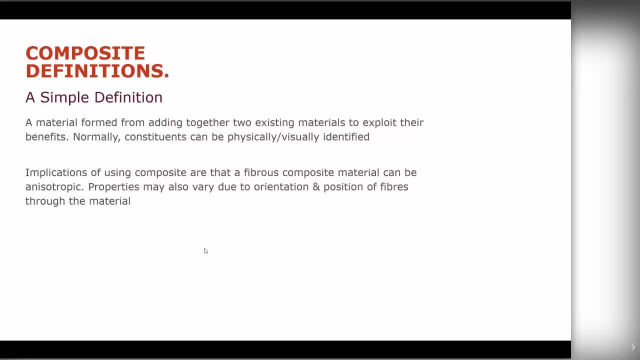 rather physical mixtures, so you can still identify fibre from the resin materials. So the implication of this is that because you have fibres that are running in a variety of directions and those fibres, as I mentioned, are rather stiff and strong- the composite materials- 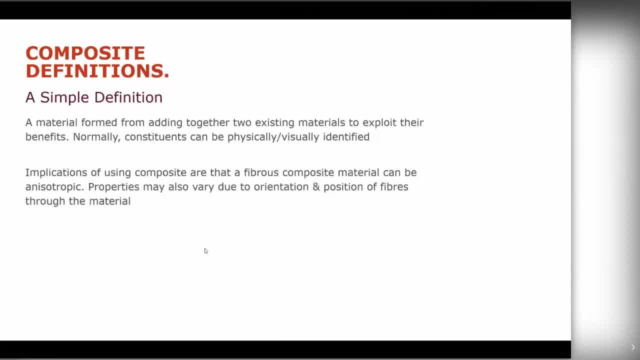 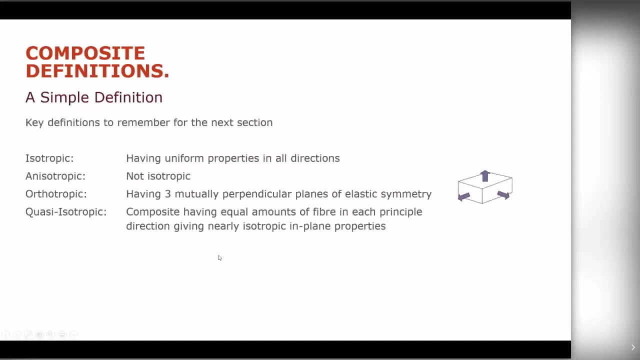 can be anisotropic. I'll talk a little bit more about that in a few minutes And a little bit more about this anisotropicity, which is quite the key, one of the key characteristics of the composite materials. So just to remind ourselves a little bit on what we mean by anisotropic – first of all, 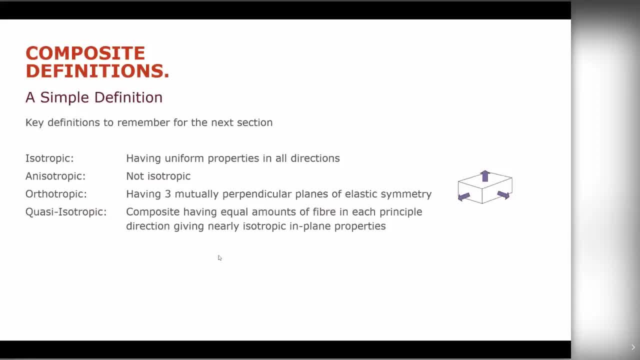 isotropic materials. typically we think of metals as being isotropic, So they have uniform properties in all directions, with little cubes to der worsell ar. the right shows what we mean by those directions. So in whichever direction you pull that material, it will give you very similar or the same response. Anisotropic material is effectively. 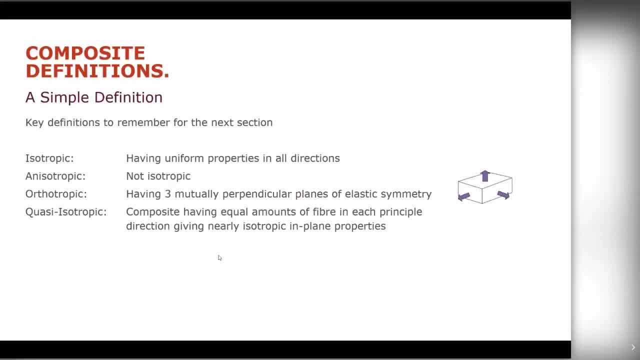 the one that has different responses in different directions. Orthotropic materials has material properties that are perpendicular along the plies of elastic symmetry- So again it will have some symmetry to it- And quasi-isotropic are. effectively, we can make composites into quasi-isotropic material by the appropriate combination of. 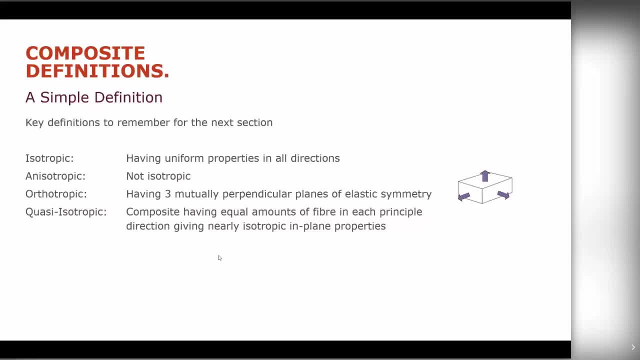 plies giving this effect of isotropicity if that is needed. But that's effectively a made-up property of the material by combining non-isotropic materials in different directions. Some further definitions. I mentioned the fibre. When we're talking about the fibre within the, 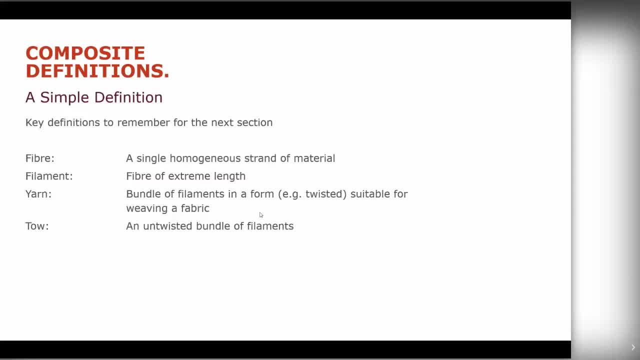 composite material. the fibre itself is a really, really thin, single, homogeneous strand of material, and fibre in itself is quite weak. That's why we typically use yarns or toes. Filaments are effectively fibres of extreme length, And the reason why we're using yarns and toes is because we're bundling the fibre. 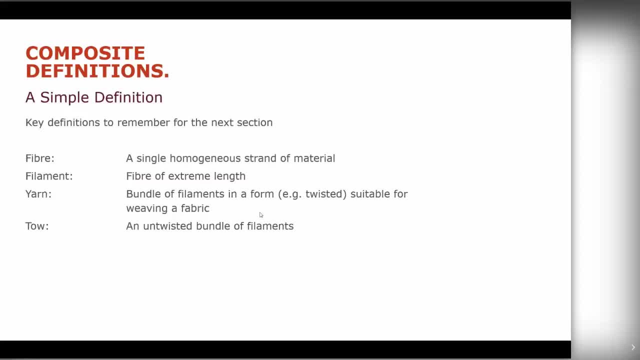 So if you pull out the fibre, or what you see as a fibre, from the composite material, you're very likely to pull yarn or a toe. So yarn is a bundle of filaments which are at micro scale bundled together and then they're suitable for weaving a fabric. 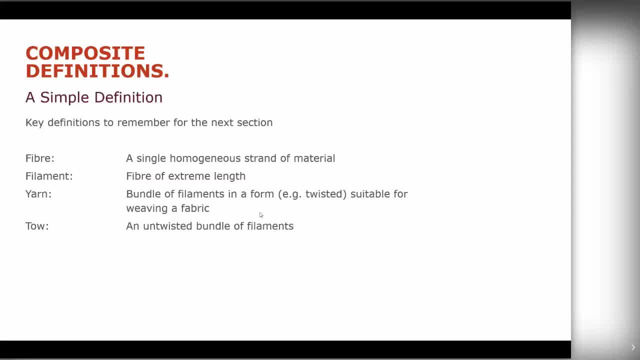 And they're also twisted. And the reason why they're twisted is, of course, processability, because it's much easier to process them. They are twisted to stay together. Toe, on the other hand, is an untwisted bundle of filaments. So these are the very basic terms of the of the fibres. 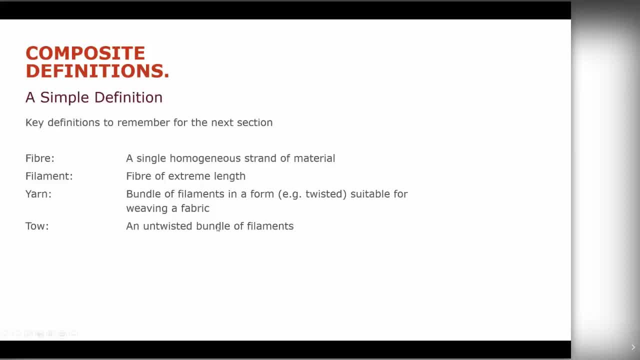 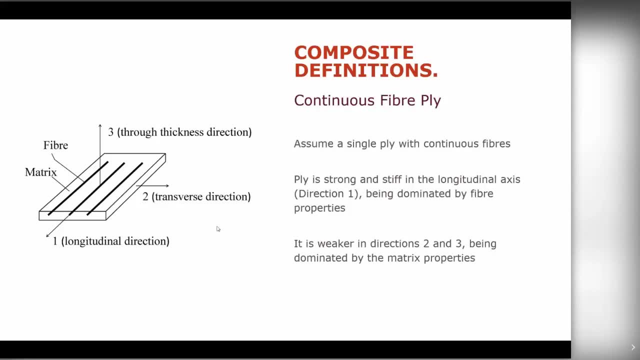 within the composite material. Okay, so now we want to bring this into a context of composite and perhaps of a single ply. So single ply is a layer of a continuous composite material which consists of fiber and the matrix, And in the picture to the left we have described some of the key properties. key: 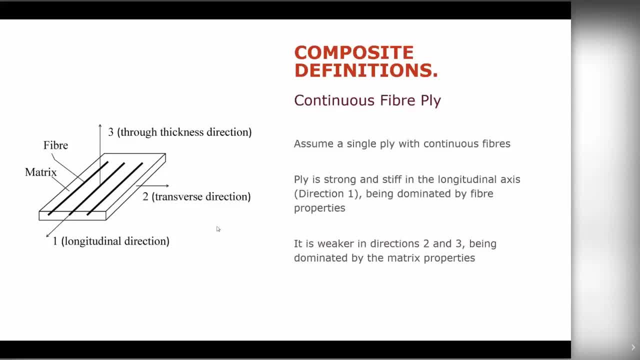 characteristics of this ply. So we have a longitudinal direction that is acting across the fiber. length Transfers is perpendicular to the fiber direction and the direction three is through thickness direction. So these are some very basic nomenclatures that define this ply. It's quite important to remember this because we'll make reference to those later on in the webinar. 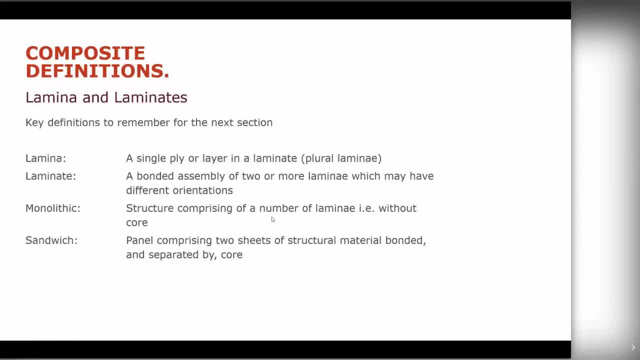 Now, further to the definitions. we talked about a single ply, which is also called a lamina, and the number of lamina make laminae. The laminae are not bonded together. However, laminate is a bonded assembly of two or more laminae, and they could have. 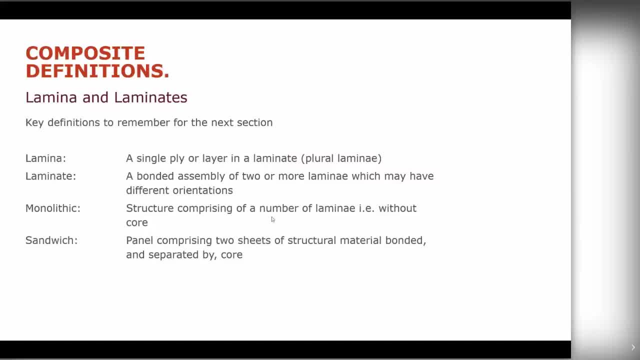 different orientations. Laminate is made out of a number of laminae or plies that are bonded together, and laminate can have number of bonds, different directions, and that orientation of different directions is something that you designers can have ability to define depending on what 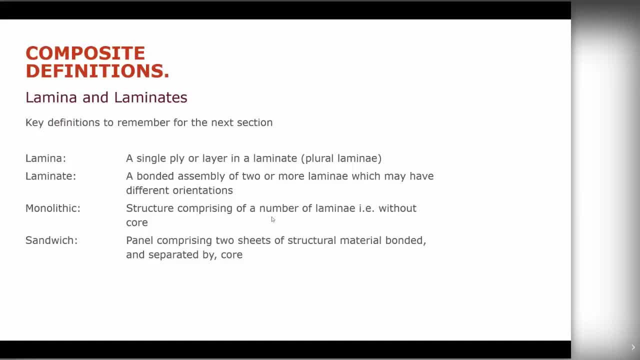 you're trying to achieve. Monolithic refers to a structure that is comprising of laminates alone. so if you have a composite material that comprises of number of plies, then we refer to this as monolithic composite structure or material. Sandwich on the other side would have a number of plies of either. 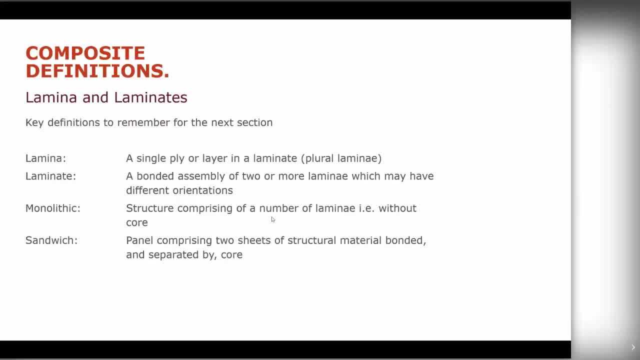 side of what they would call a core material. So it's a panel with two sheets which are effectively bonded to the core that sits in in the middle, effectively adding to the second moment of area to resist bending better. So that's really what the sandwich is. 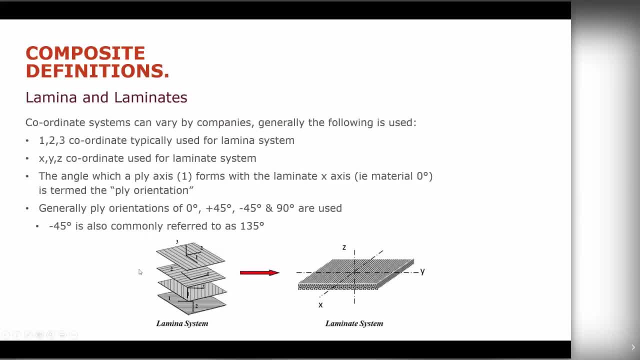 Okay, so I mentioned some basic terminology, starting from the fiber filament, yarn and tow, representing the key structural component of the ply. This is mixed with resin to make a continuous ply. We also mentioned that each ply has their own set of directions that are very useful because, along the 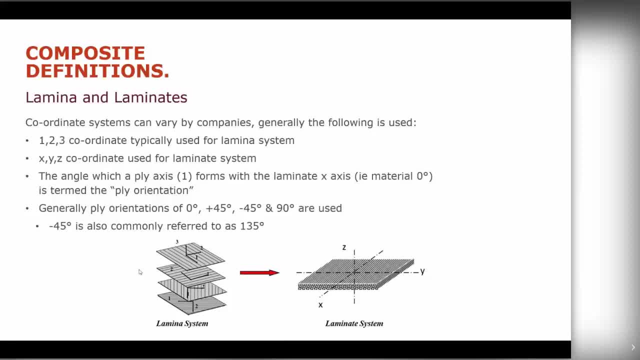 direction one is dominant stiffness and strength. Direction two is characterized by effectively resin properties, because what holds the ply together is the resin, And the direction number three is through thickness. We also mentioned that the laminate is made out of lamina, so you can see in the picture at the bottom of this slide. 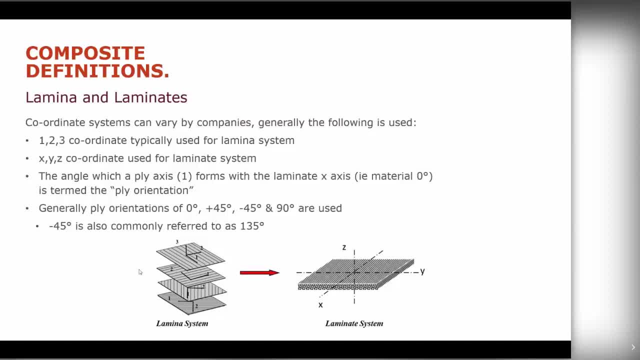 a number of lamina that are unconnected with their own orientations: one, two and three. One always aligns with the fiber direction. Two always is perpendicular to the fiber direction for each of those laminae. One goes through laminas or plies, and three goes through thickness When they bond. this 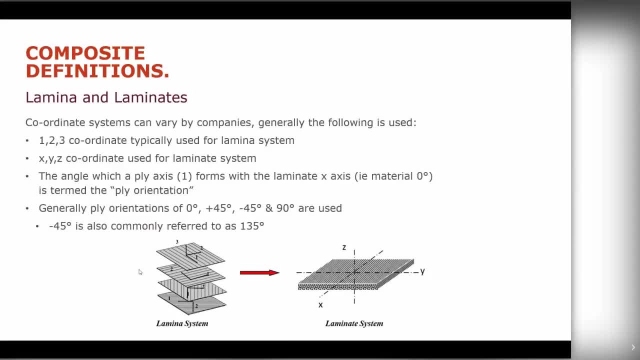 assembly of lamina or plies together we get laminate, And each laminate depending on orientations of individual plies, we have different properties depending on what we are trying to achieve. So one, two and three are coordinates typically used for lamina systems, whereas x, y and z's. 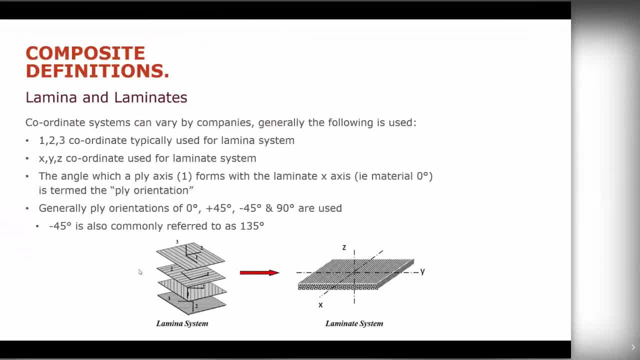 are typically coordinates used for laminate system And we generally in composite manufacturing would use simplified number of angles, orientations for plies, mentioned here as 0,, 45,, plus and minus and 90s, to aid easy ease of manufacturing. So we can get the same results. 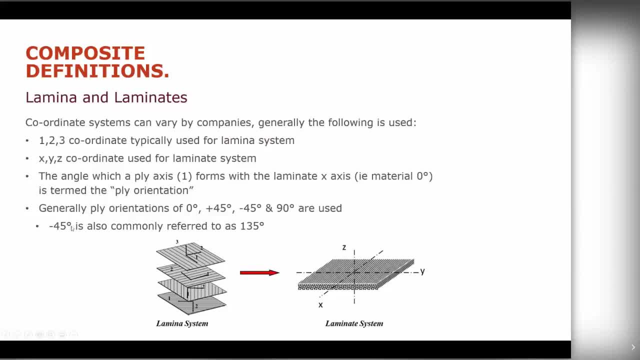 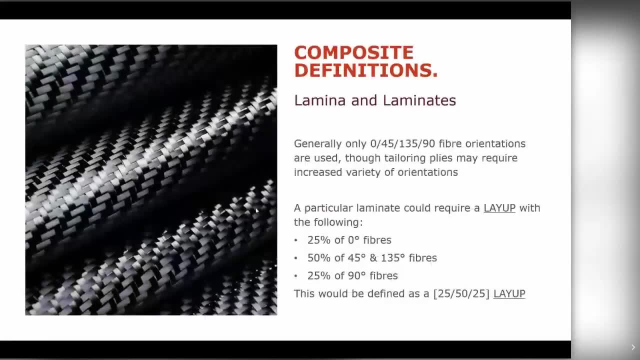 So we can get the same results. And sometimes minus 45 is also referred as 135 degrees And sometimes minus 45 is also referred as 135 degrees. So I mentioned that generally we only use 0's, 45's, 135 and 90 orientations, because that 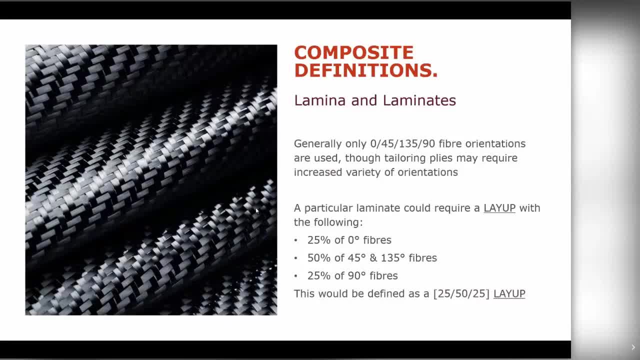 enables ease of communication between design and manufacture and, of course, aligning those fiber directions on the manufacturing shop floor becomes easy. Further, to communicate this between design and manufacture, some simplified methodologies have been devised. So, for example, if your laminate consists of 25% of 0 degree fiber, 50% of 45 and 135, 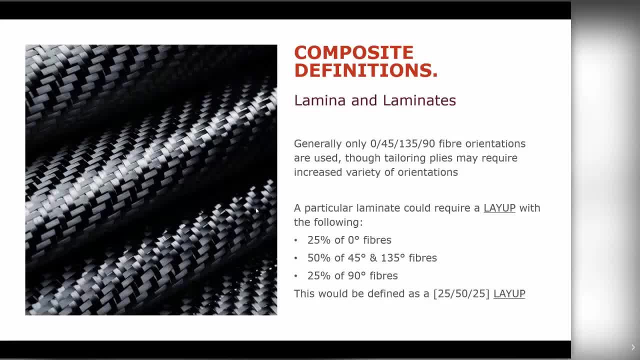 and 25 and 90,. you could use a nomenclature presented at the bottom to present the whole layup. With this nomenclature you wouldn't necessarily know how the design is going to look like, So you could use a nomenclature presented at the bottom to present the whole layup. With this nomenclature you wouldn't necessarily know how the design is going to look like. So you could use a nomenclature presented at the bottom to present the whole layup. With this nomenclature you wouldn't necessarily know how the design is going to look like. 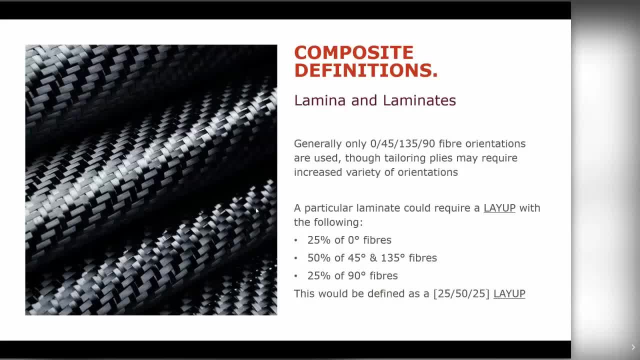 So you could use a nomenclature presented at the bottom to present the whole layup. And if you had no idea how the plies would be distributed in the stack, you would know that you will have 25% of 0,, 50% of plus minus 45, and 25% of 90 degrees fiber. 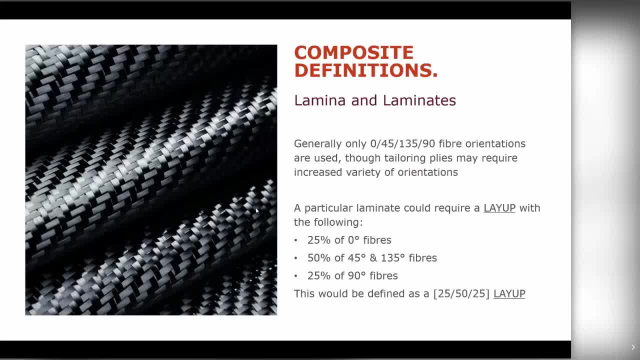 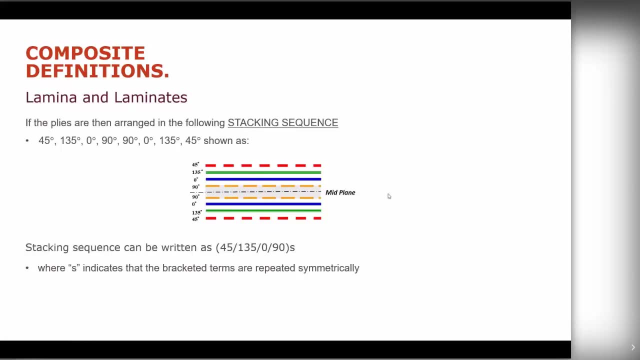 But this would be perhaps sufficient for some structures to be manufactured or the information communicated between the design office and the manufacturing shop floor. So if you're to define a design, you have a number of components that we have to use. define your composite a bit further. you would need to define something that we call a stacking. 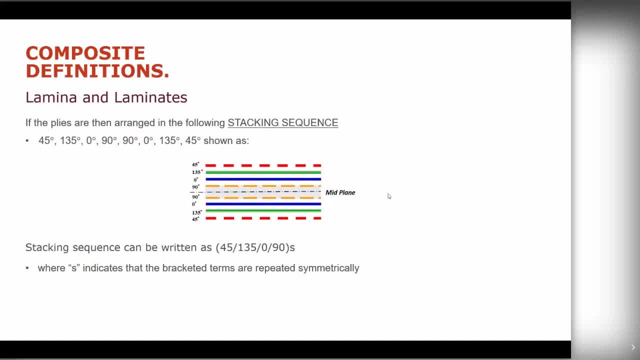 sequence. So in this case, you can see the picture in the middle representing each ply with a different color and the weight of the of the line. So what we have here is a symmetric stacking sequence. What it means is that along the mid plane, represented by the dashed line, 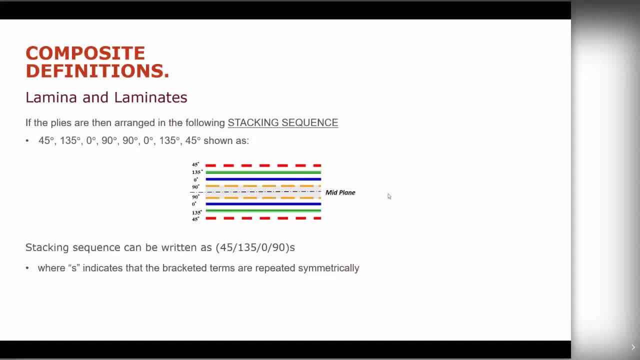 you have effectively a mirrored picture of the top segment of the stacking on the bottom, and this stacking sequence could be only represented with one side from the mid plane or along the line of symmetry. So you can see 45, 135, 0 and 90 in brackets, followed by letter s. 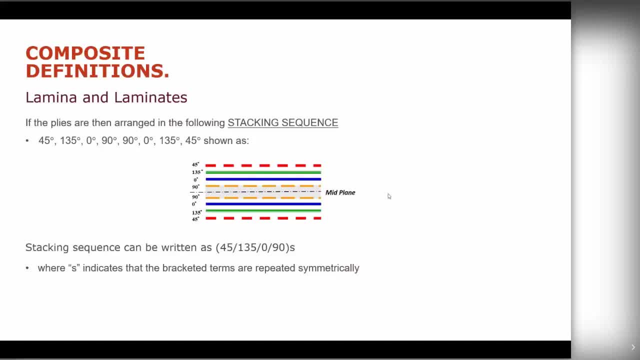 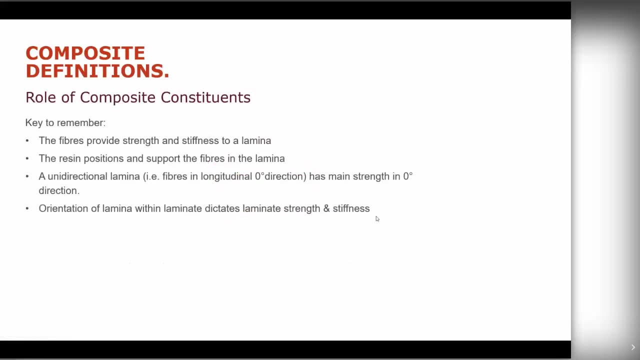 suffix, which represents it is a symmetric stacking sequence. So this is another nomenclature that is sort of used in the design and manufacture of composites. So just to reinforce the message I mentioned before, the reason for having fiber is to provide strength and stiffness to the lamina. 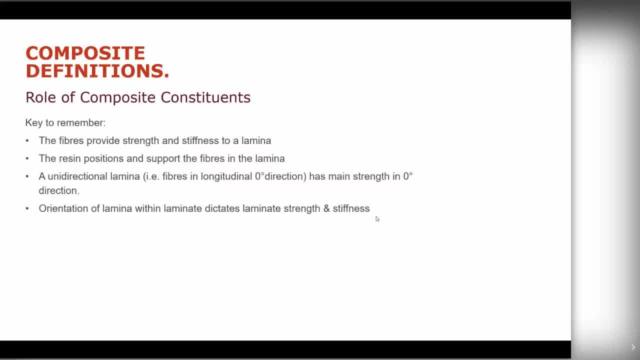 and the resin is used to keep those fibers together and to position them in the right direction. Unidirectional lamina, or the lamina that has a fiber only in one direction, has the main strength in zero direction, and that is because that fiber really acts in that direction. 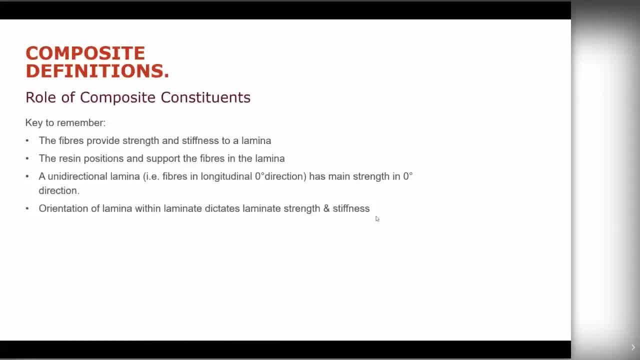 And then orientation of lamina with the laminate will determine the strength and stiffness of the of the whole laminate, and this is where you, as a designer, will have a a freedom to find what works best. and this is where the composites are really useful, because you could then tailor each and every part of the structure to resist only what is necessary. 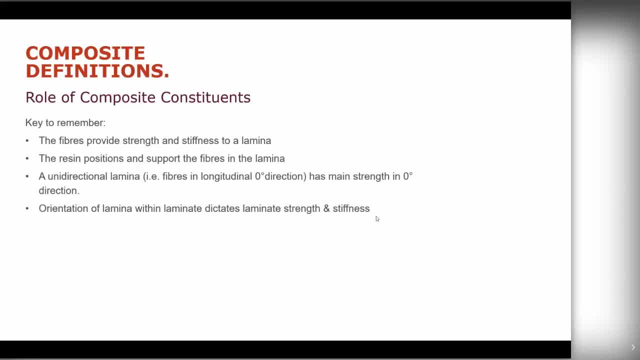 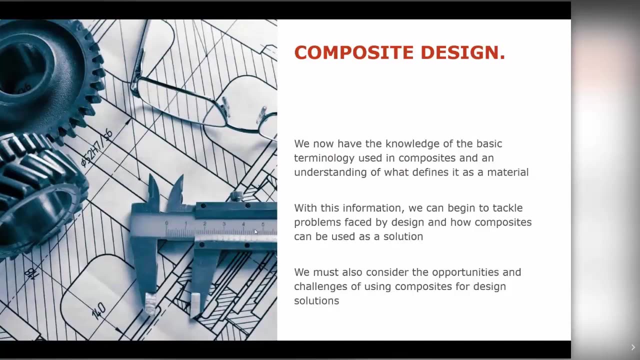 hence reducing the weight and reducing the material needed to support the operating environment. Okay, so this was a sort of a very, very brief crash course of the composites terminology and of course, there is a lot more that needs to be learned. This is only intended to give you some indication of 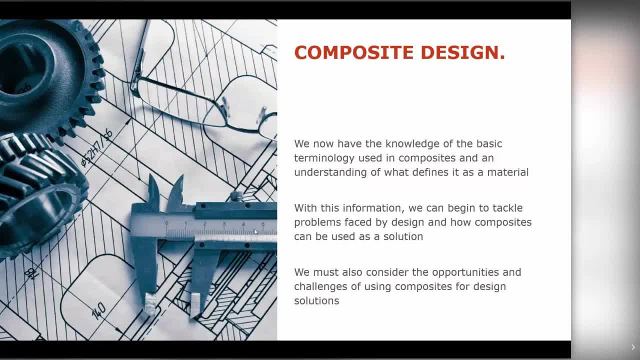 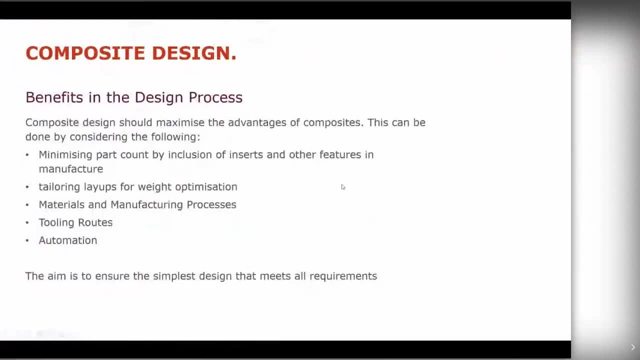 what the terminology and what the constituents are to be carrying out design. but this would be enough for now to make an introduction into the topic of design and how to approach designing with composites. So just before we start talking about designing with composites, um, I just want to uh again reinforce the message. Why do we want to design with composites? 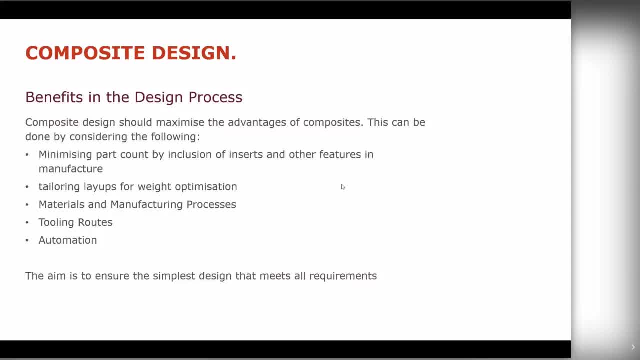 There are benefits, of course, uh in using composites and those benefits are mentioned. this in this slide, because composite material uh is effectively made at the same time as when the part is being made. you can incorporate in your composition, such as bisschen parts, or you can've. 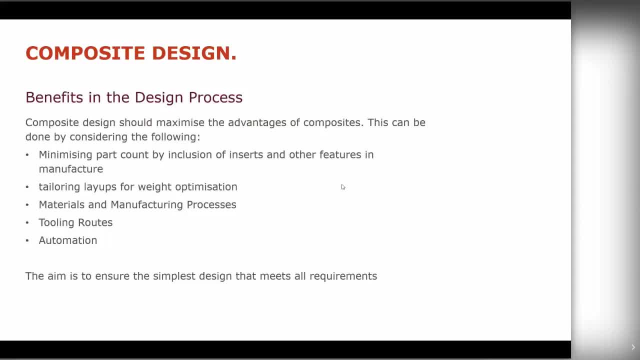 incorporate in your component a variety of features that otherwise would need to be manufactured separately and then bonded joint or whatever, So you could end up having minimized path count. So that's one of the benefits that could be explored or exploited if that is your design goal. 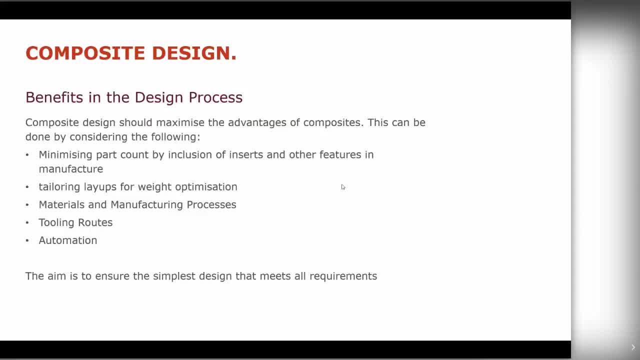 You could tailor your layups for weight optimization. I mentioned that you, as a designer, will have freedom to look at orientations of different zones and reduce the weight and number of plies to only what is needed. You can choose appropriate materials and manufacturing processes to bring some functionalities that your composite part might have. 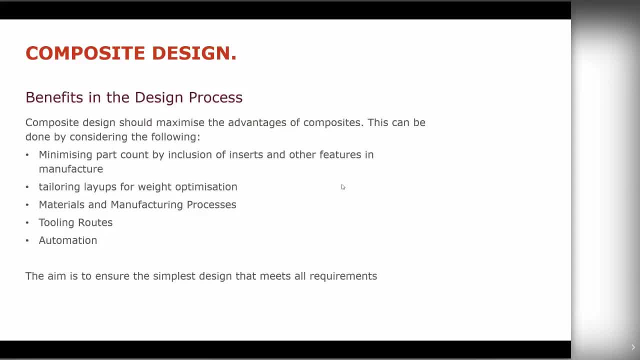 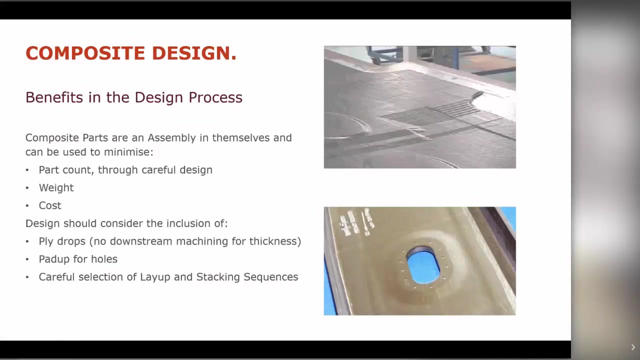 You can consider a variety of tooling routes depending on the rate of production And finally, you can consider automation effectively if your part needs to be made in a larger series. So I mentioned before that you could reduce path count through careful design and also weight and cost. 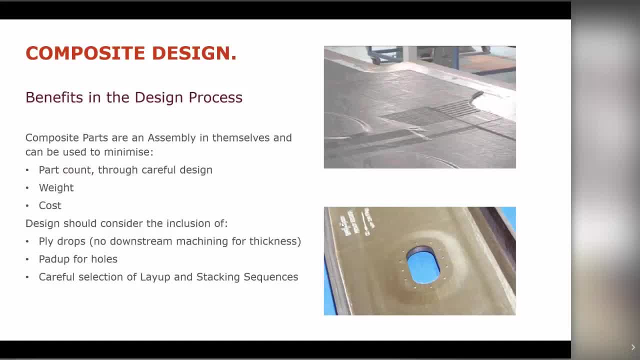 And you can see the picture to the top right. You have a typical scale. You have a skin that has a variety of zones And you might notice that some zones are thicker than the others. There are some ramps in this picture, represented by slope between the thicker and thinner zone. 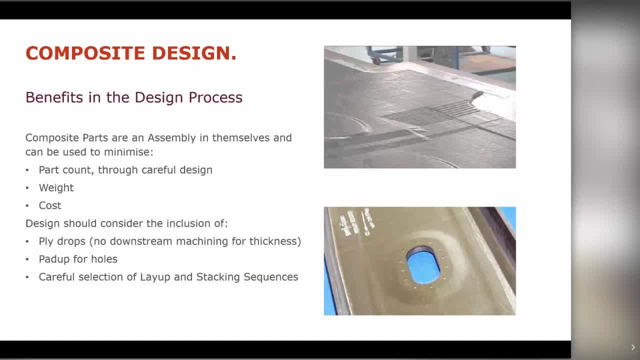 And the reason for this is because the thicker zones are designed to react high load and the thinner zones are designed to react lower load. because it was found that the thicker zone sees high load, And this is where you can actually reduce weight and consequently cost, because of course, you are using less material in a particular zone. 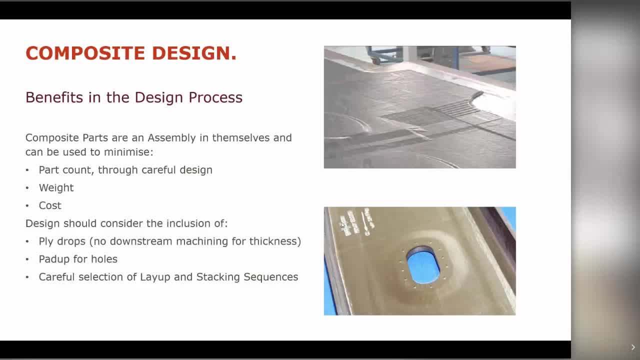 So this is how you would realize that particular benefit, And your designs need to consider a variety of features, because, of course, composites react slightly differently to the environment than the metallic counterparts, So those ply drops will need to be designed rather carefully so that the load transfer between those plies is appropriately achieved. 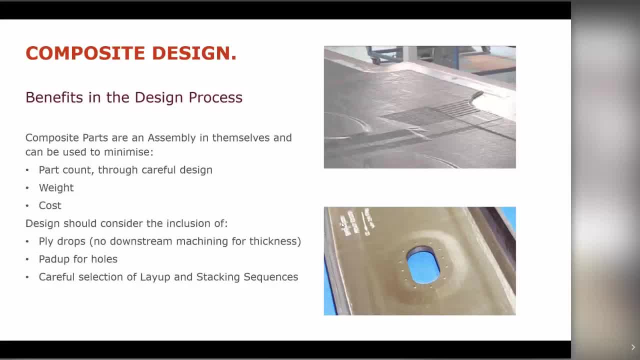 The paddocks and holes are another feature that will affect your design And, of course, you will need to be carefully designing and selecting labs and stacking sequences, And we'll talk a little bit more about this. There is not enough time in this webinar to talk about all of these topics. 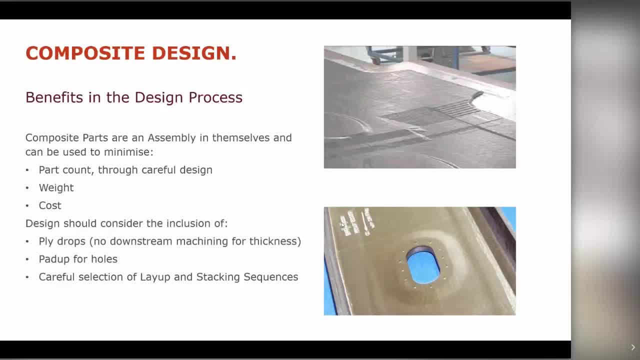 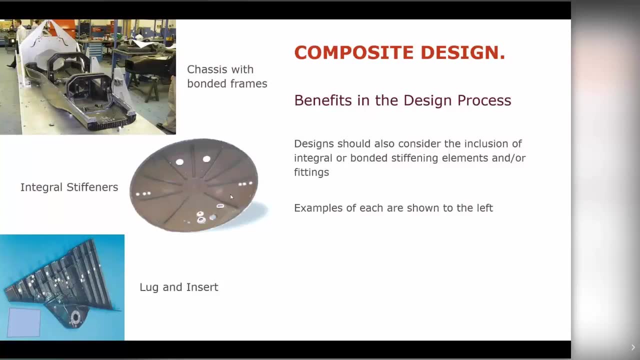 But we mentioned some of the very typical design guidelines, Design rules that help designers come up with some of the products. So, further to the considerations mentioned before, designs should and can consider inclusion of integral and bonded structures so that we can reduce part count. 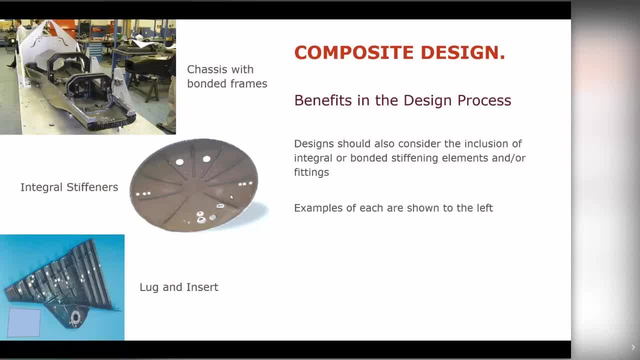 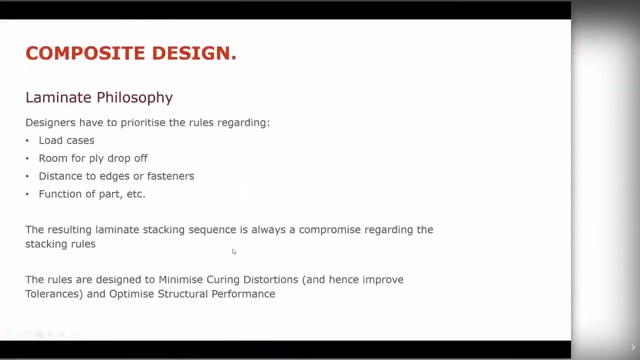 And you can see some examples here where structures are effectively singular structures. If they're made out of metal, you would need to have each piece machined separately and then bolted together, which could be heavy and introduces a number of additional operations on the manufacturing shop floor. 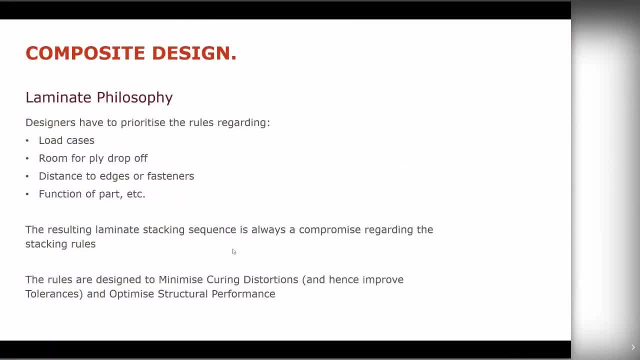 So, in terms of creating laminates or designing for using composites, designers will need to understand load cases. They will need to understand the geometry within which they will have freedom to operate to allow for those ply drops. If there are bolted joints to be created, distances to the edges and fasteners are quite critically important. 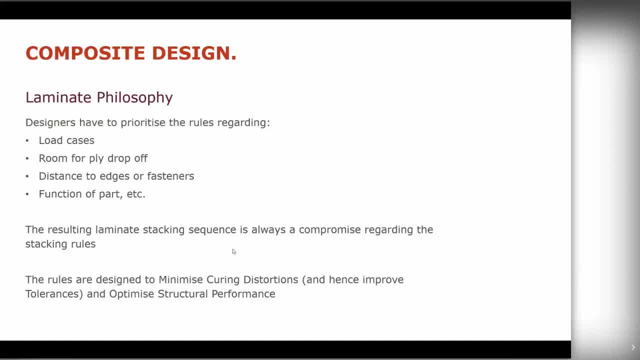 The function of the parts. So there is the whole list of criteria that designers will need to consider in order to achieve the appropriate results. And, finally, your design will always be a compromise of those criteria, because if you're really strongly pushing for one particular criterion, 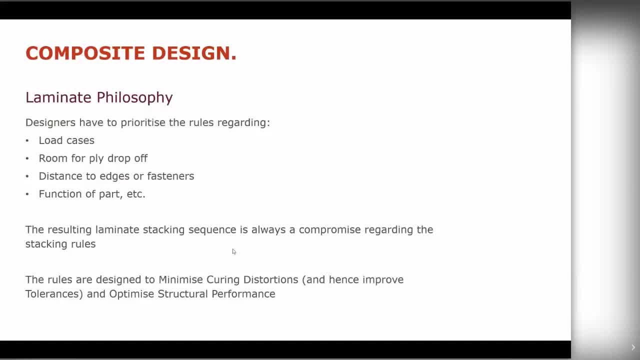 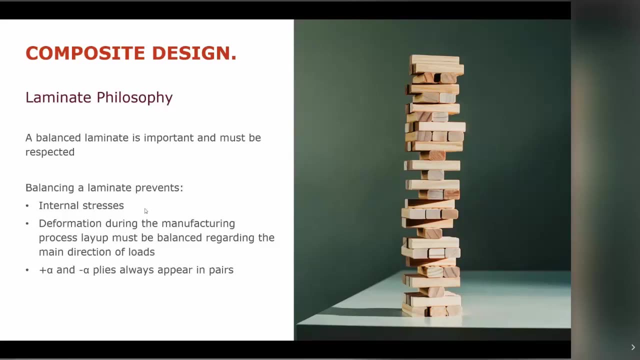 some of the other ones might be compromised. So it is an iterative process to effectively achieve our optimized and compromised design. So one of the key things in designing is effectively achieving a balanced laminate. A balanced laminate is when you have across your stacking sequence. 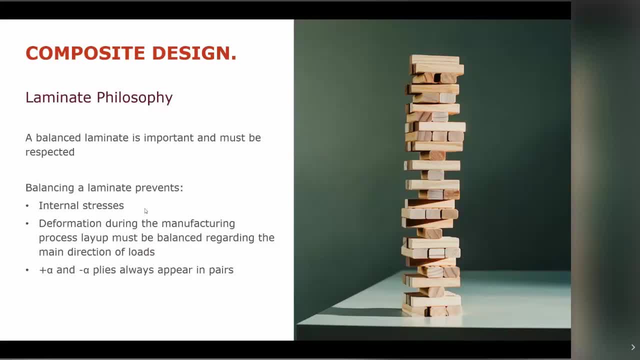 equal and opposite side of positive and negative orientations of the ply direction. So, for example, if above and below your symmetry line you have equal and opposite number of plus and minus 45 plies, Then that would be considered having a balanced laminate or balanced stacking sequence. 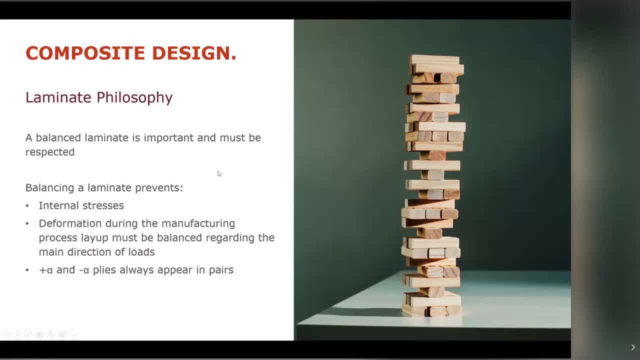 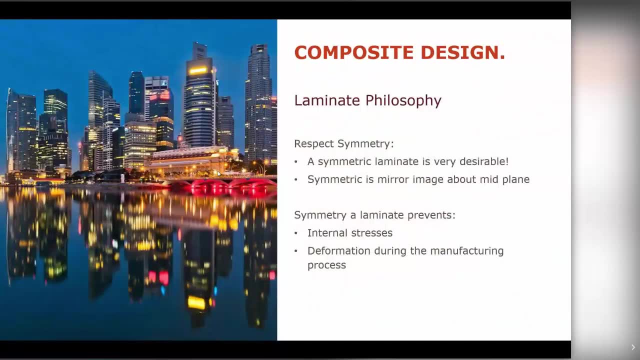 And I will show you a little bit later why is that important. Another rule that designers typically tend to obey is symmetry. So having a mirrored image of your stacking sequence above and below the line of symmetry And combined with the balanced rule, you effectively avoid having internal stresses. 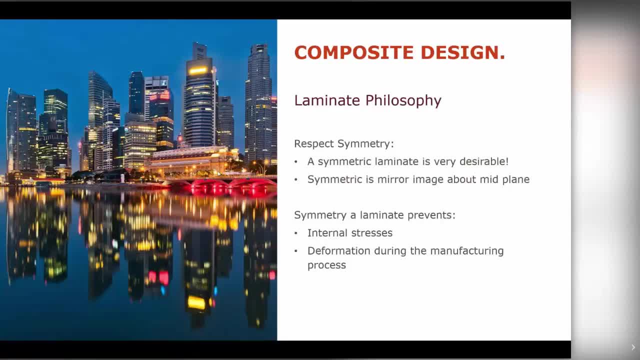 And the logic is very simple. If your laminate above the line of symmetry is reacting load in a particular way and that is not mirrored below, you have some imbalances in how load is being reacted in your structure effectively, causing some of these effects. 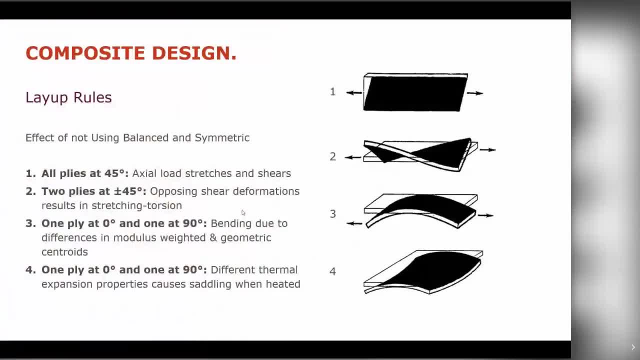 So it is very interesting to see these things And I have seen them in practice. when designers design unbalanced or unsymmetric structure, You, after the cure and demolding of the part, end up having a part that is effectively deformed because of those effects. 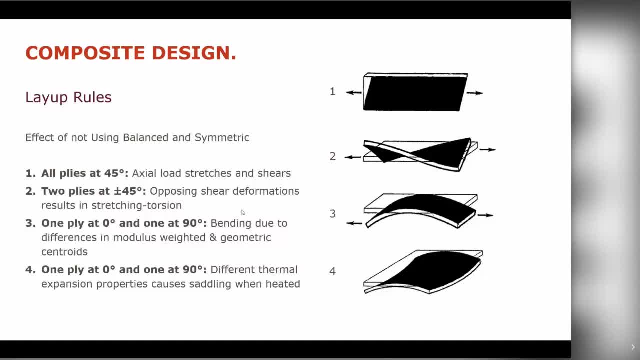 So this is why, typically, you would tend to avoid having unbalanced and unsymmetric structures. I do have to say that sometimes, in particular fields of engineering, these designs are actually desirable And you want to perhaps utilize this for your aeroelastic tailoring, for example. 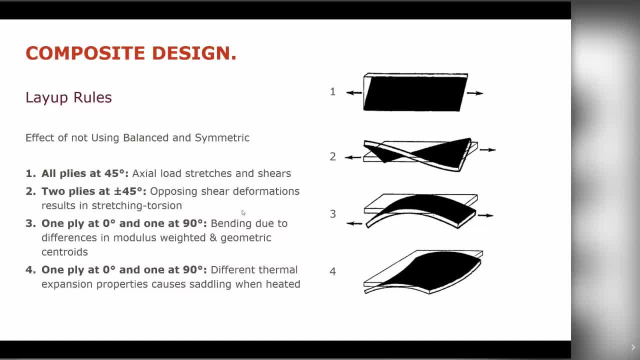 where the load case and the load imposed on a structure would cause your structure to orient itself into the most optimized position, But those would be very high-end applications. For the majority of engineering applications, you would tend to design it as symmetric and balanced. 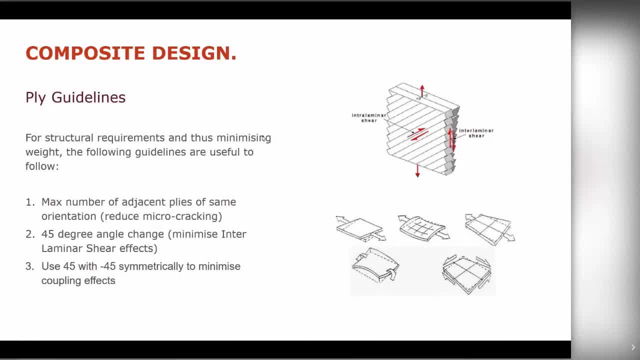 So these are some of the generic design philosophies. There are further design guidelines that I will mention here. They have been invented as a best practice by engineers and started by NASA in the 60s. So they're sort of mentioned here And I'll talk over them. 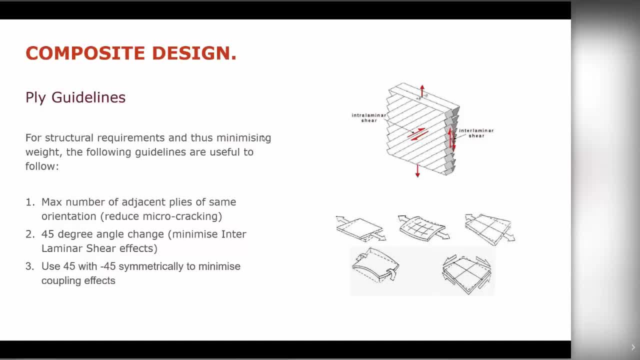 So you are tending to avoid having a number of plies in the same orientation stuck next to each other because there is nothing to react load in the opposite direction, causing some micro-cracks. If you do need to change ply orientation, tend to stick with 45-degree change because that's a minimum change in the load path. 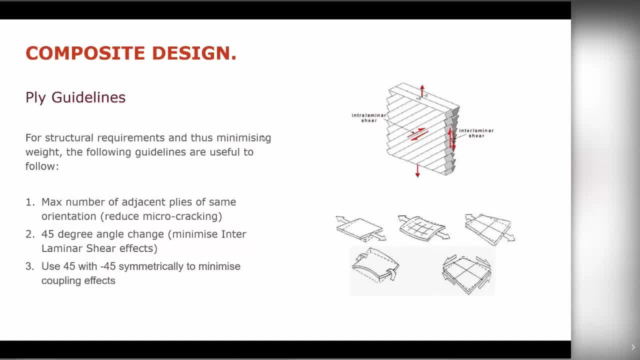 again reducing the interlaminar load. Use 45s with a negative 45 symmetrically to minimize coupling effects. That's in line with what we talked about before. You would need to have at least some amount of any direction: 0, 45, minus 45,, 90,. 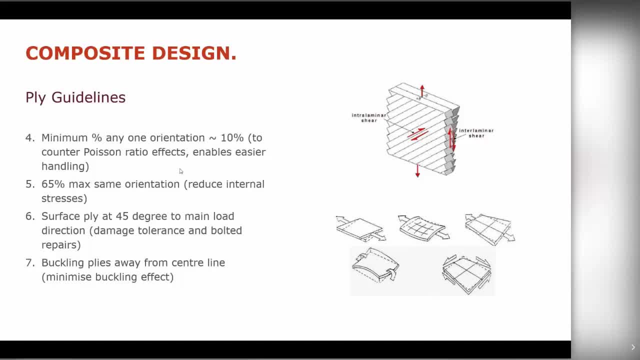 let's say 10%, to counter for personal ratio effects and also to counter for linearity. Also, to counter for some of the additional uncated load cases, Maximum number of orientation in a single direction should be no more than 65, although I have seen examples where this rule has been compromised. 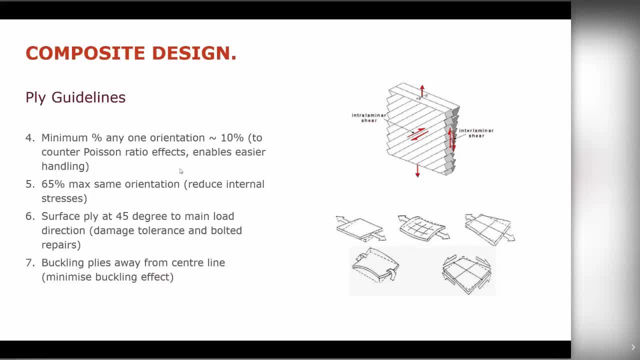 This is the design guideline that you are trying to stick to. to start with, You would tend to stick to plus or minus 45 degrees plies at the surface To prevent any damage to the structure And any buckling plies. that's effective with 0 plies should be away from the centerline. 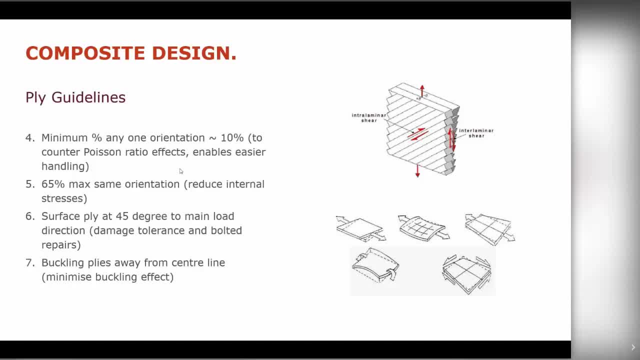 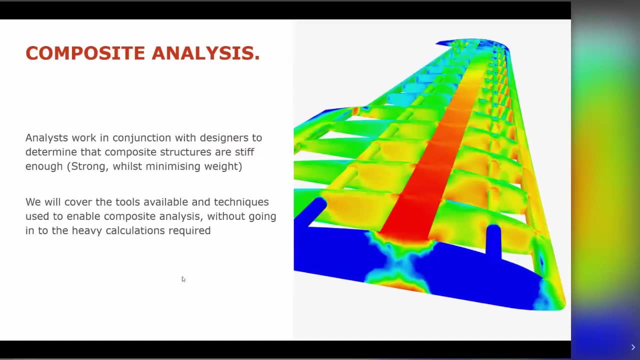 because you want to minimize the buckling effect by creating a larger distance from the centerline and effect the second moment of the area. So you can start to see that the complexity of designing this model with composites is great because we are having this huge design freedom. 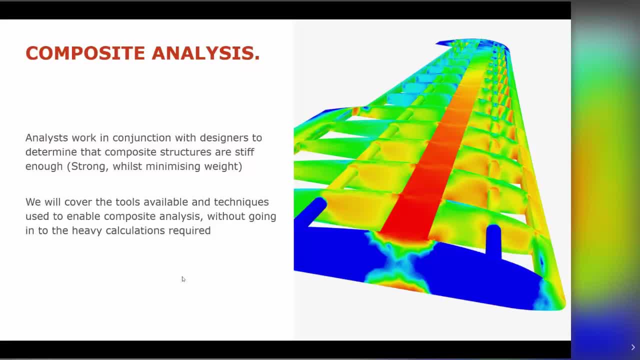 And just by me talking over some design rules that are created to help designers generate good structures. there is a huge amount of design analysis and it is a very iterative process, And this is where we actually start to use some additional tools to actually analyze composites. 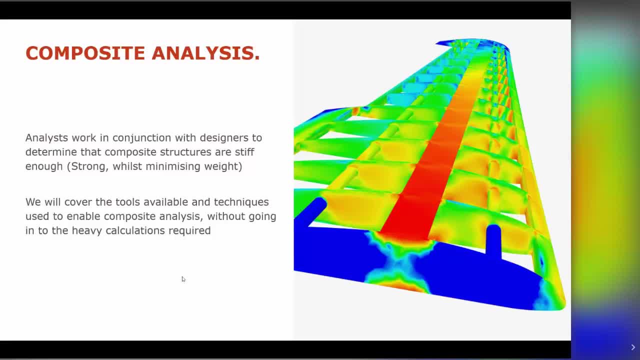 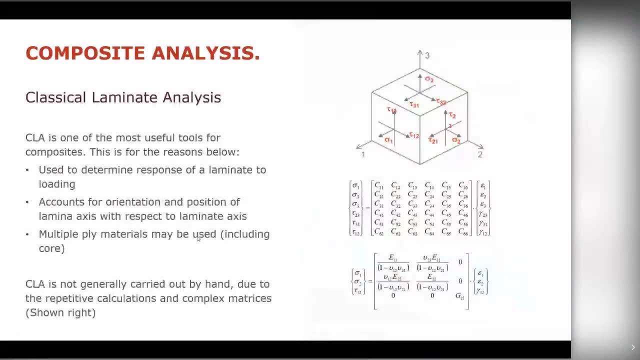 because design rules will give you probably a very good first stab at this, But then you will need to run some more involved analysis. So in this particular course we will very, very briefly touch upon classical laminate analysis, because it is quite an involved mathematical procedure derived to actually analyze composites. 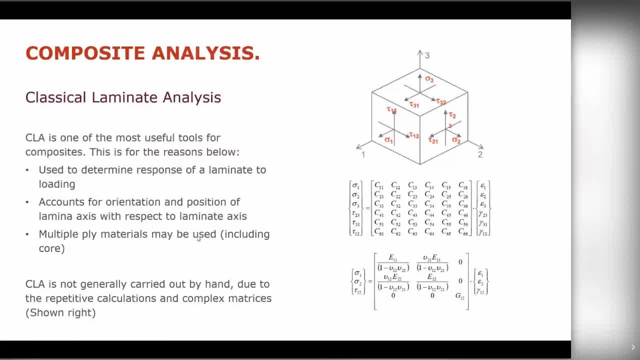 to analyze structures And it will help you to find the strengths and stiffnesses and failures of composites. And I will not even attempt to go through the mathematics of it now, But what it does? it will enable you to find the stiffnesses and strengths and failures along your composite. 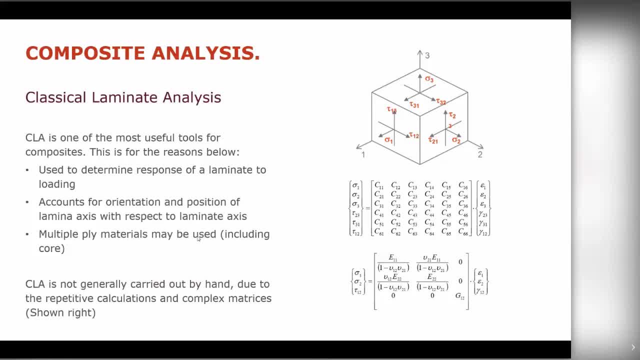 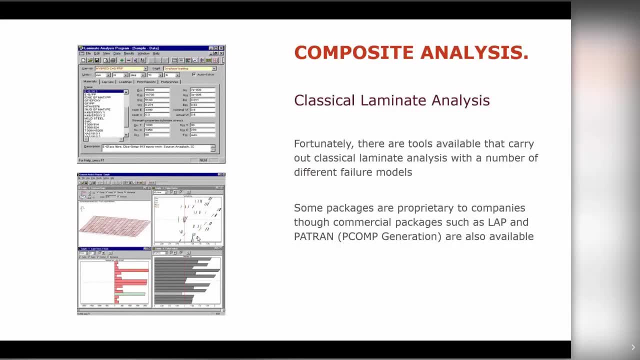 through thickness for each ply. Luckily, there are tools that exist out there that will help you in carrying out these analysis that are fairly involved, And this is one of them presented here, called LAP, But also many modern finite element programs such as PATRON or others. 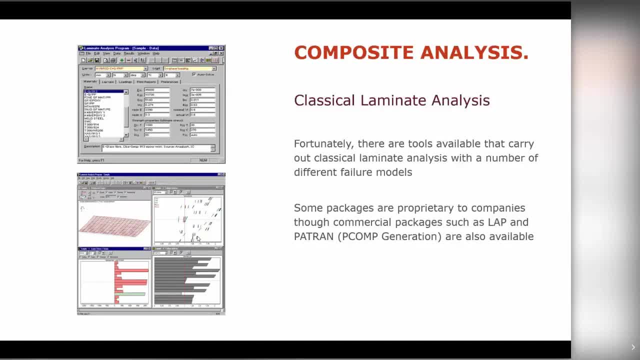 would have, effectively, an instance of laminate analyzer built into them to cater for analysis, The analysis of the composite materials, And they will also take care of all the ply lamina, laminate orientations, transformations of loads and so on. But you would need to be careful. 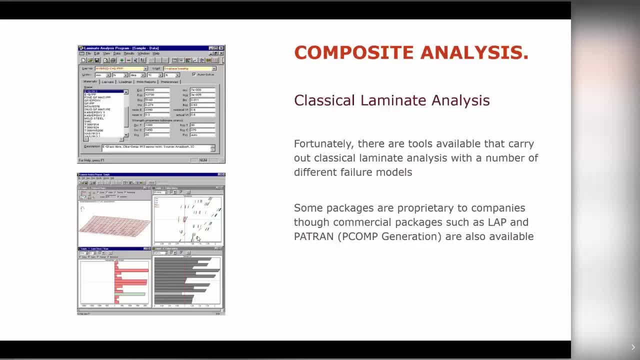 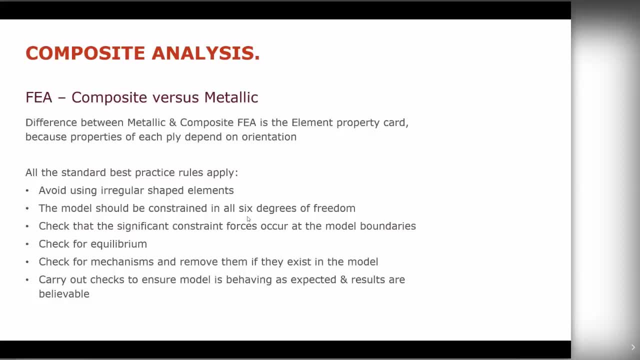 You would need to be trained separately to actually be able to use this in an appropriate fashion. So ultimately, you would use finite element modeling tools as your composite materials, And for composite materials, the material model is different to the metals, Because each ply depends on orientation. 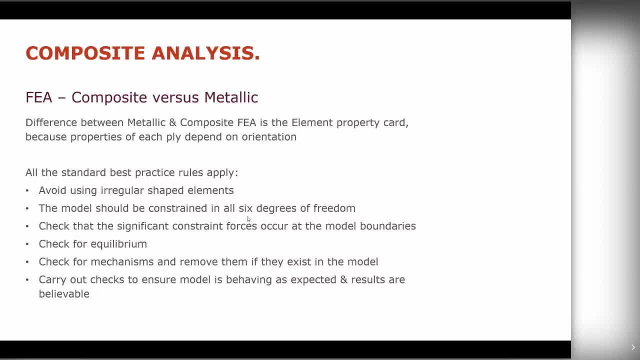 So there will be a separate module in each finite element tool to actually cater for this. When you're doing your design in a finite element analysis tool, all the best practices would apply anyway. You'll just have ability to run your analysis in a bit more streamlined or easier fashion. 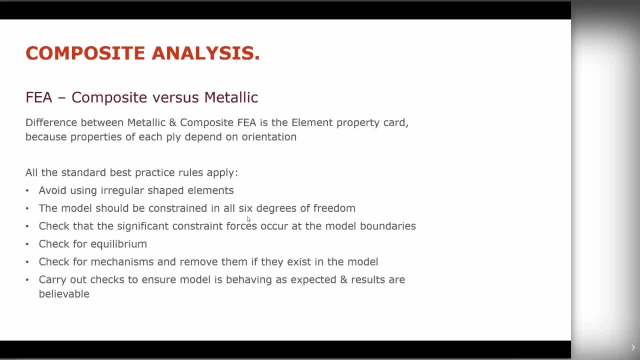 But there are some rules of what you should try to avoid, which generally do not differ from using finite element analysis in any case. So you should try avoiding irregular shaped elements, Models should be constrained, You should check for equilibriums, And so on. 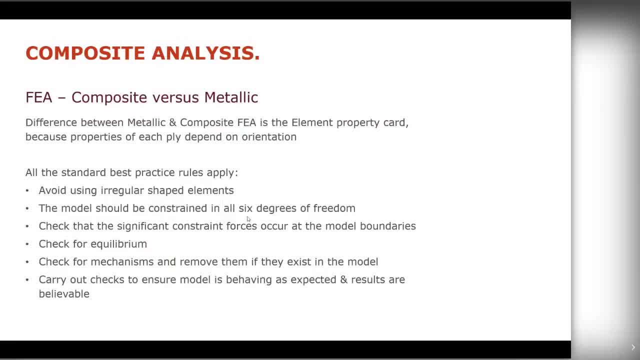 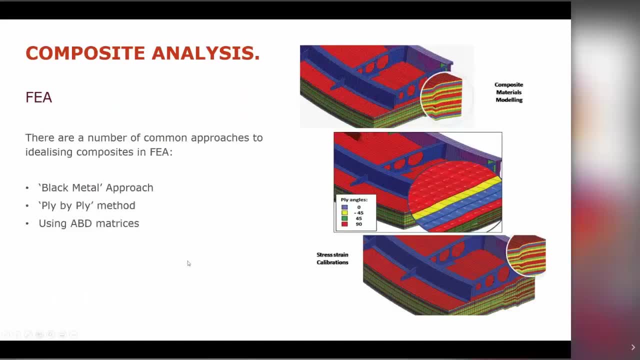 So effectively, basic rules of building finite element analysis model would be applicable. So when you're building your finite element model, there are a number of approaches that you could apply. So there is a black metal approach, Ply, blight, Ply by ply method and using ABD matrices. 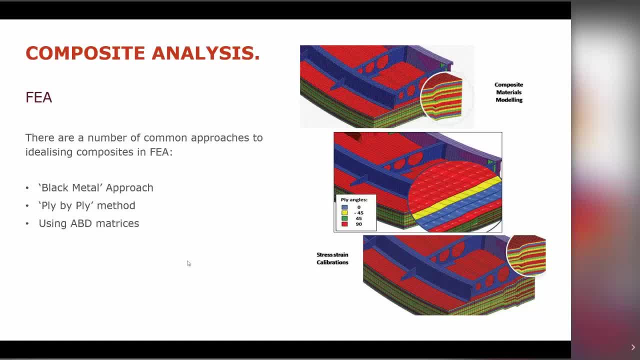 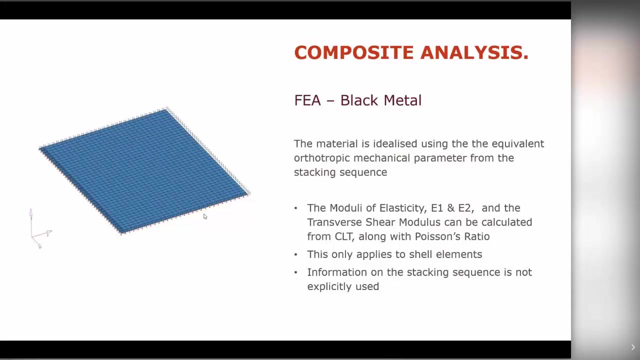 And you remember from the slide talking about classic laminate analysis. ABD matrices are constituents of the laminate analysis. So, one by one, the black metal approach would effectively consider the whole composite material and its architecture, ply by ply, as a single slab of material with equivalent properties in all directions. 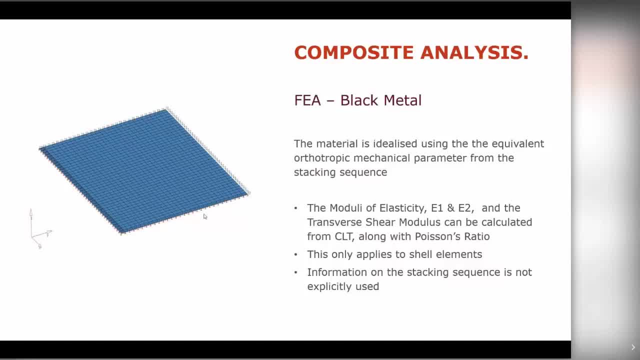 So the software would actually calculate what is the effective properties in X, Y and Z based on laminate. So you wouldn't be able to see the interaction between the plies or how the failure indices distribute through thickness. You would get a failure for the whole slab of material. 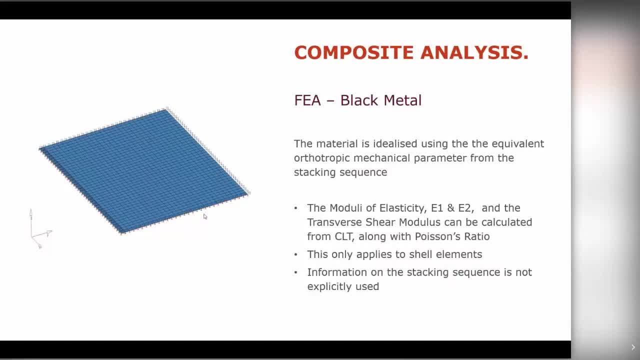 And this is a very useful methodology. So this is a very useful methodology when you're doing initial conceptual design, because you don't have enough time to iterate around the number of plies, But it is restricting you in actually optimizing the structure or getting the maximum out of your component. 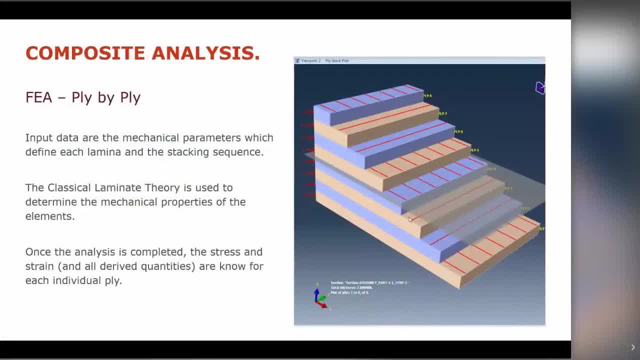 On the other hand, ply by ply approach would require quite detailed input into finite element model, where you would model each ply separately and input the definition of ply in terms of material and the orientation and the stacking sequence, And this approach would actually give you quite a bit of details. 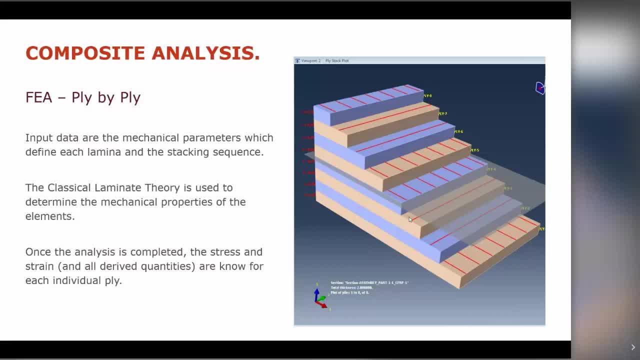 of the behavior of your structure in terms of stiffness, strength, failure indices, interlaminar behavior and so on. And just to summarize, Just to touch very briefly because this is quite a deep topic You could go into 2D ply by ply approach. 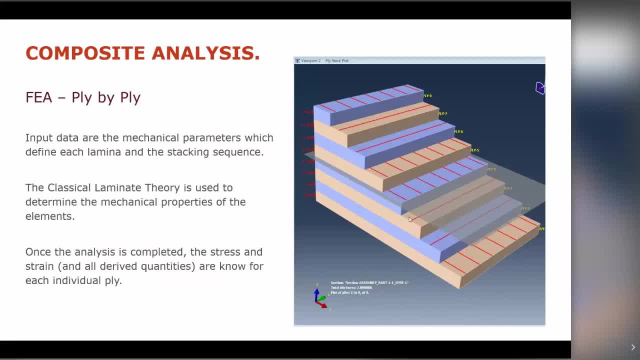 which will give you some approximation of the through thickness stresses. But if you really are worried about the through thickness behavior, then you would probably be advised to model it as a 3D solid part. Of course that comes at an expense because that's quite an involved procedure. 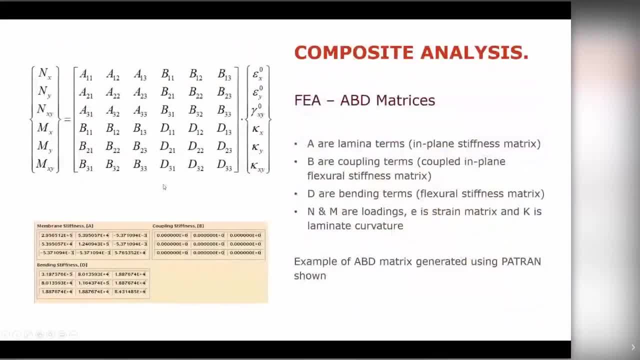 And finally, you could use the ABD matrices approach. For this. you would need to compute those ABD matrices by using classical laminate analysis And effectively plug those back into your finite element modeling tool. That will enable a rather quick turnaround of the 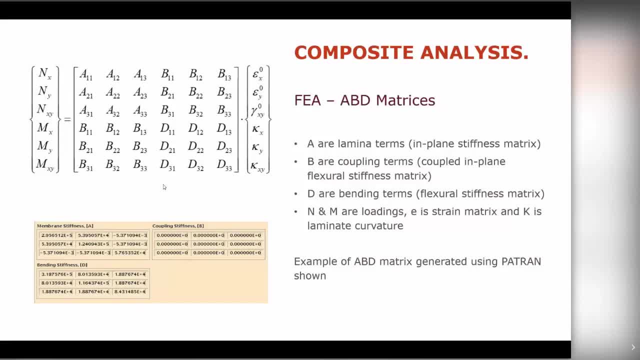 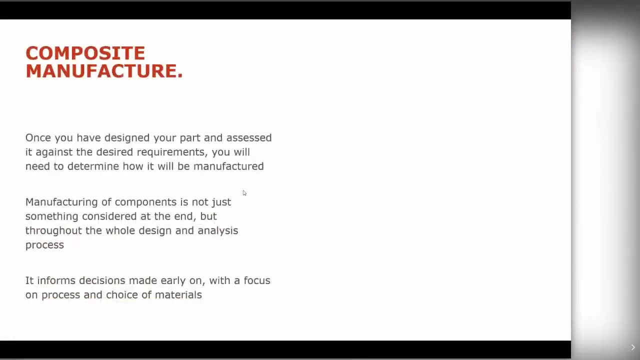 of the analysis, And you would probably need to do some additional analysis outside of them to transform the results into each of the of the plies, But that would be entirely, entirely possible, Right? So I'll give you a very, very, very brief introduction of analysis. 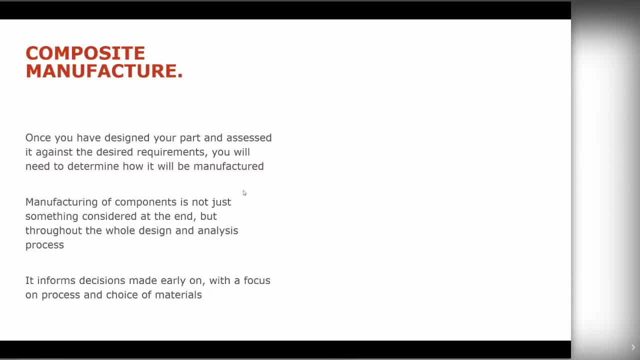 of composites and the complexity associated with the design freedom, Because we can choose material in terms of resin and fiber, We can choose fiber orientations in each ply And then we can choose fiber orientations across a number of plies, And all that needs to be. all the complexity needs to be somehow analyzed. 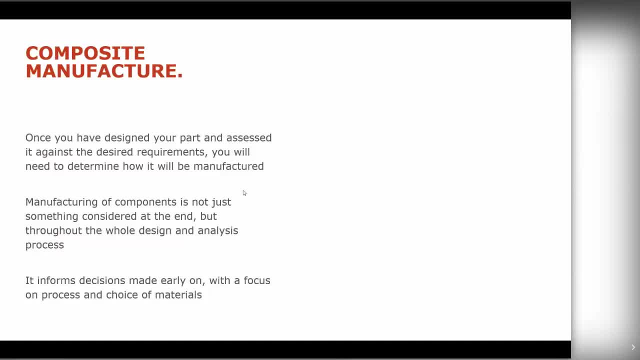 And typically we would use tools. We would use some design analysis tools to do so. But that's not the only complexity of composites. Actually, manufacturing in itself is a quite complex topic, And this is where the interaction between design and manufacturing needs to happen. 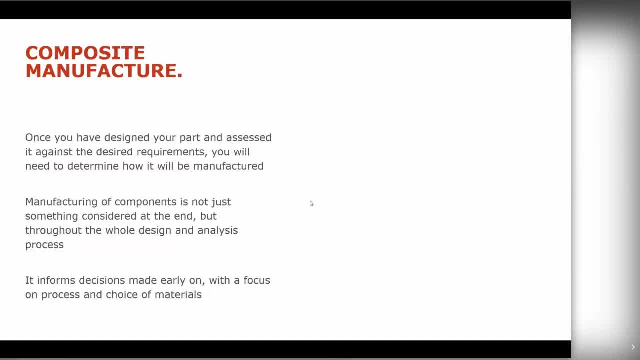 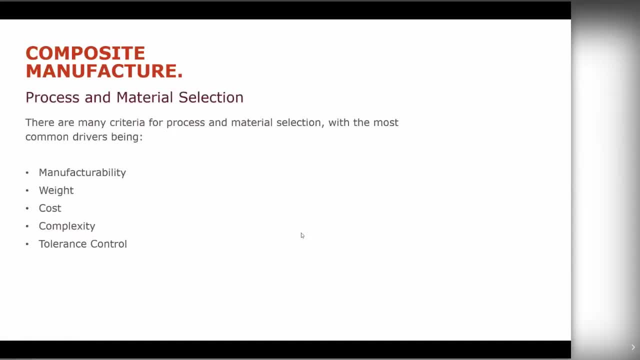 Because otherwise you might end up with non-manufacturable parts. So typically, before you start manufacturing or developing a part, you need to think of some criteria relevant to your particular use case, But manufacturability is one of the things you need to think about. 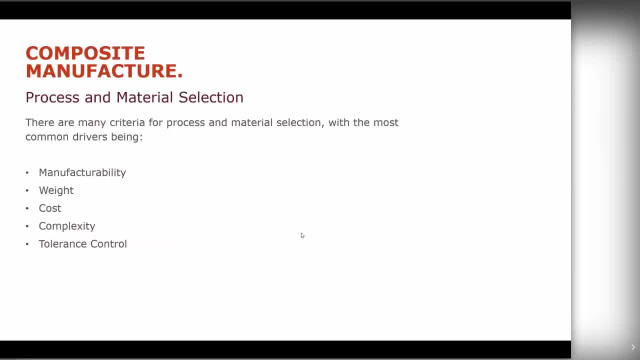 Weight might be a criterion that you need to consider, Cost almost certainly Complexity of manufacture, of assembly of perhaps even transportation sometimes, because we are making rather big parts, So transportation might be a significant design criterion- And ultimately, tolerance control. So how do you assemble parts and still stay within the prescribed tolerance level? 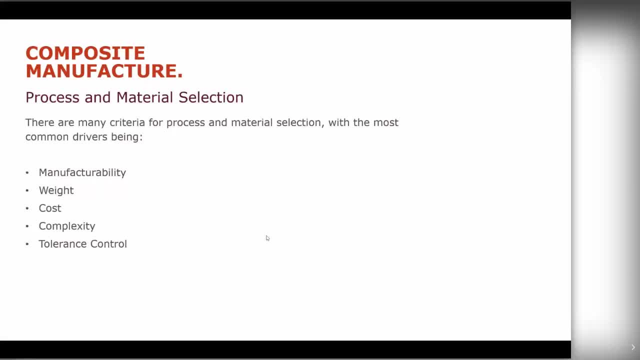 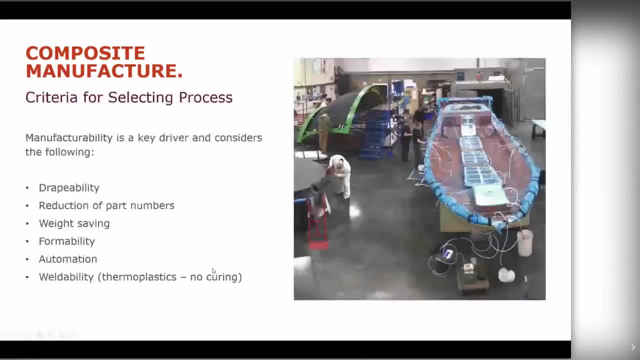 And all of these things will need to be considered And there will be a strong interaction between design and manufacture activity in achieving those criteria. Okay, so how would we select the process? Well, we mentioned some criteria. of course We would need to consider, for example, 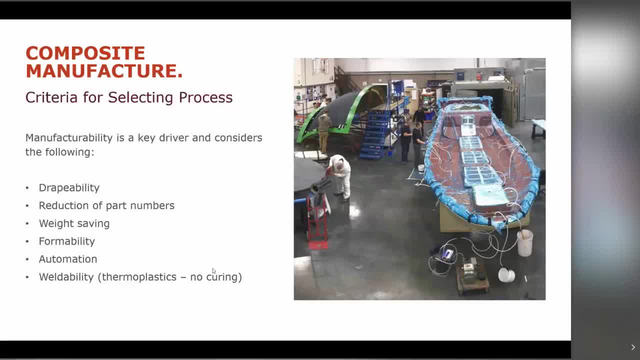 if you're making one-off or ten-off, the number of parts will play a significant role in your choice or manufacturing process. The manufacturability, which is sometimes represented as drapeability- How does the fibre and the material drape forms around a particular profile? 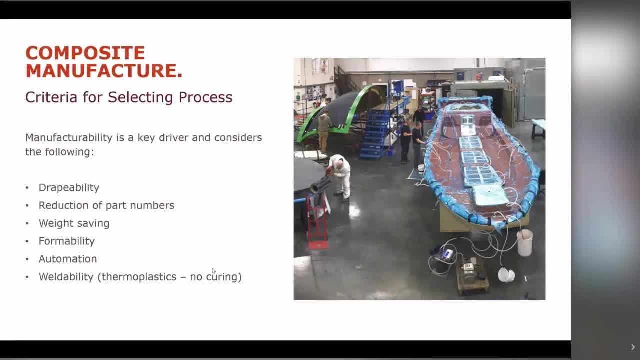 Can you save some weight? Can you form the part? Is automation applicable? Can we use, for example, welding as opposed to curing in case of thermoplastic? So these are all the considerations one would need to make before choosing the appropriate manufacturing process. 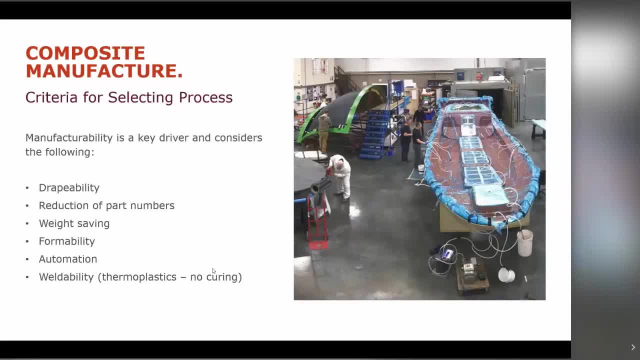 And typically conceptual. design or study would be carried out with a selection matrix that would rate pros and cons of a variety of manufacturing processes across different criteria to figure out which manufacturing process would be the best. Another thing is, of course, with some manufacturing processes. 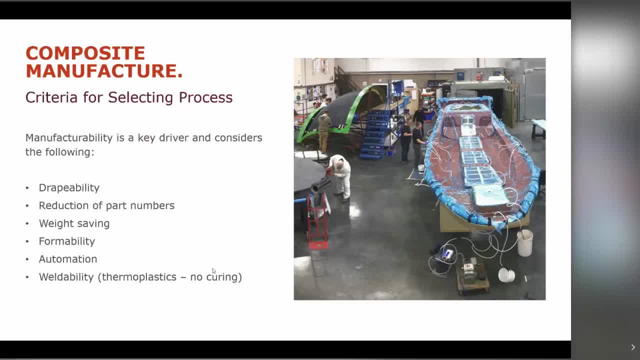 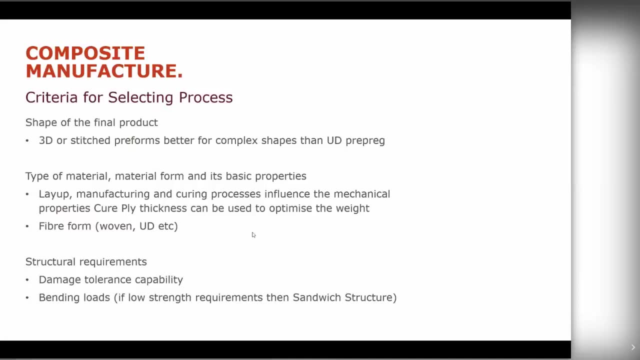 achieving particular design features might be more or less possible. So if that is important for a particular part, that might be a criteria that drives the selection of a particular manufacturing process. So here are some examples of how that might affect the selection. So one of the manufacturing process or preform creation process. 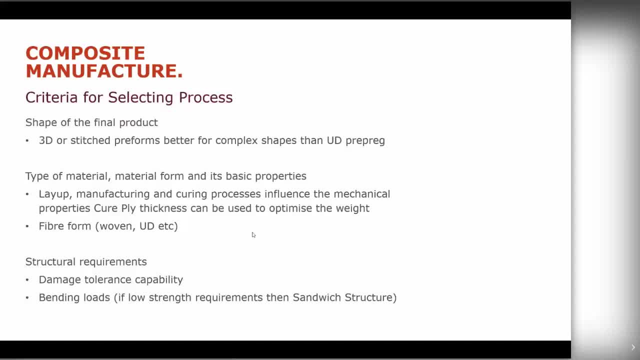 is the selection of 3D or stitched preforms that are better for complex shapes than UD prepregs. And that's quite simple, because UD would actually drape or form differently to those complex shapes. So, type of material, material form and its basic properties. 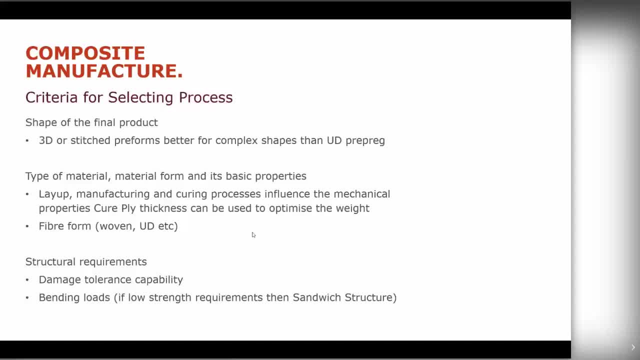 also affect the criteria for selecting processes, Because they would affect the mechanical properties. cure, ply thickness, which then affects the tolerancing and overall design, will need to be considered. And, finally, structural requirements will need to be considered because, of course, composites need to be damage tolerant. 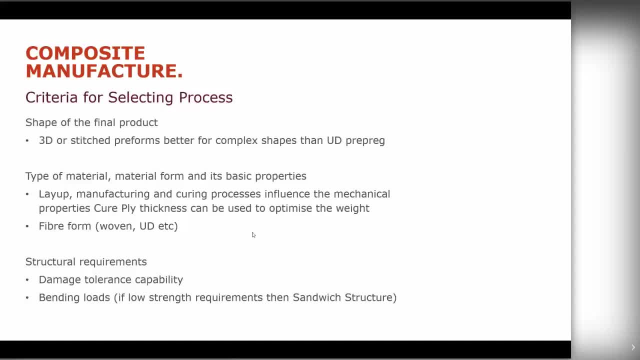 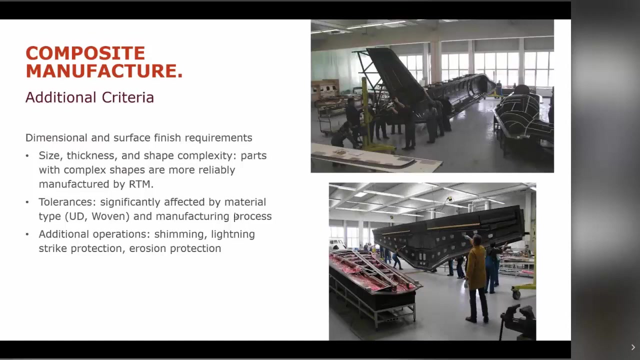 and perhaps they will need to withstand bending loads but sometimes impact loads, So you would need to think about how to integrate features inside your composite material, composite part that will enable that impact absorption. Some of the additional criteria, So dimensional and surface finish requirements. 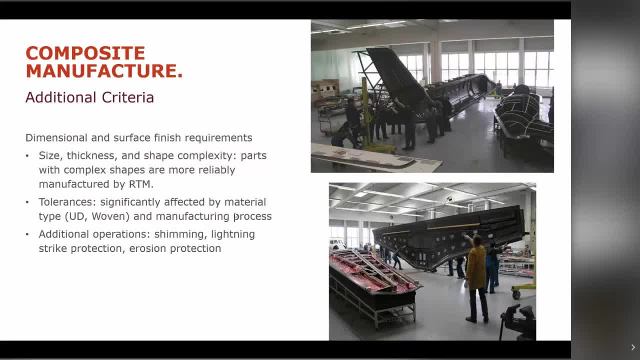 So, for example, if you are developing a part for automotive sector, surface finish is absolutely critical. Assembly In aerospace is again another very, very critical characteristics, And the size, thickness, shape and complexity of these parts influences the choice of manufacturing process. 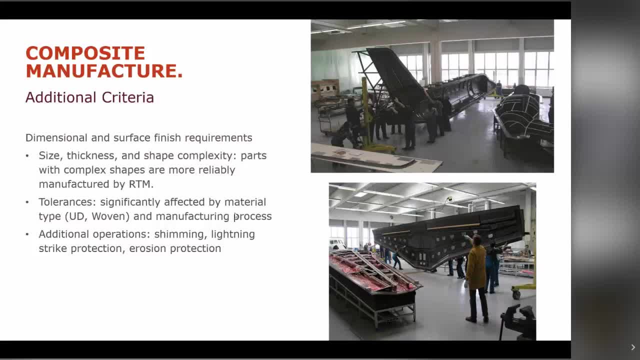 I do have to remind that the composite manufacturing is still heavily manual, And the repeatability of the part to part manufacture is something that needs to be particularly taken care of, And therefore the selection of manufacturing process might be limited to only few processes. 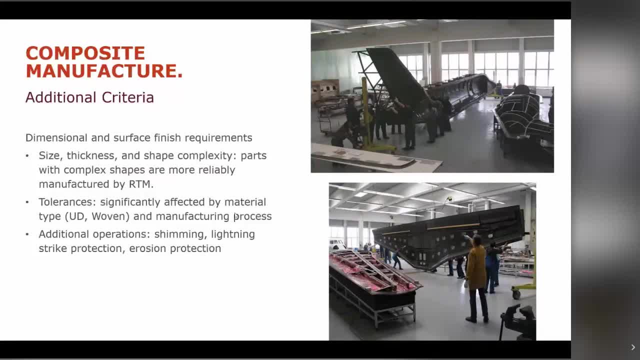 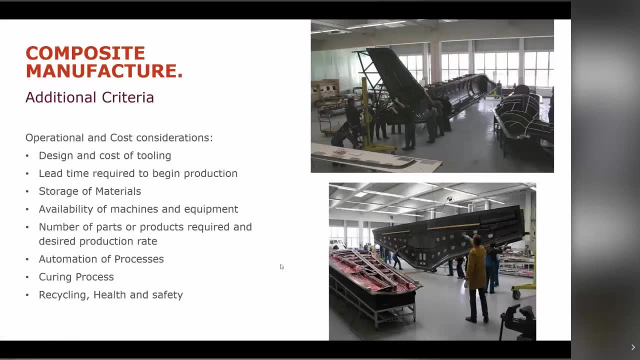 if this is the key criteria for the selection, Of course there are some other criteria, such as shimming lightning, strike protection, erosion protection and so on and so on. I mentioned tooling. Ultimately, the tooling is a large part of the cost. 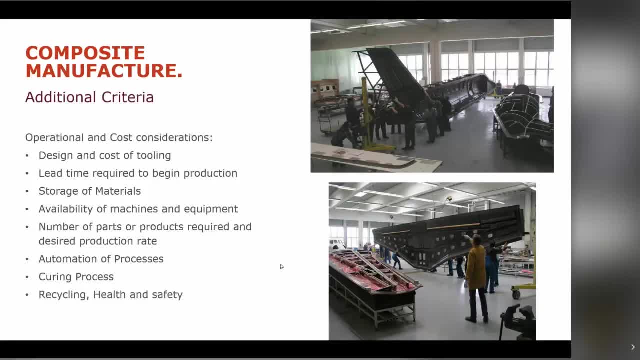 And one would need to consider that rather carefully, because if you're making only one part, you probably need to be thinking how to recover that cost of tooling through making only one part. If you're making a number of parts, then the tooling could be recovered. 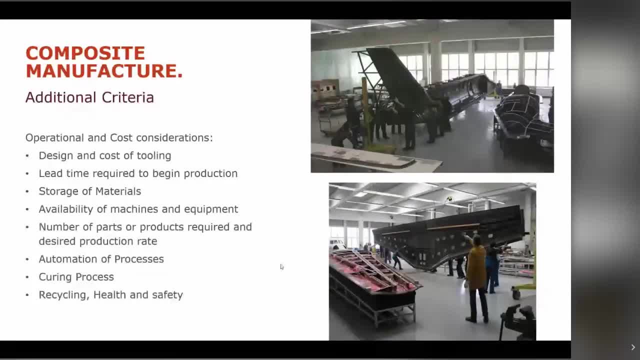 through a serial production which gives you ability to think about maybe more expensive option for the tooling. So that's the solution for the tooling which enables easier manufacturing. Some very pragmatic and practical things might need to be considered. Lead time required to begin production. 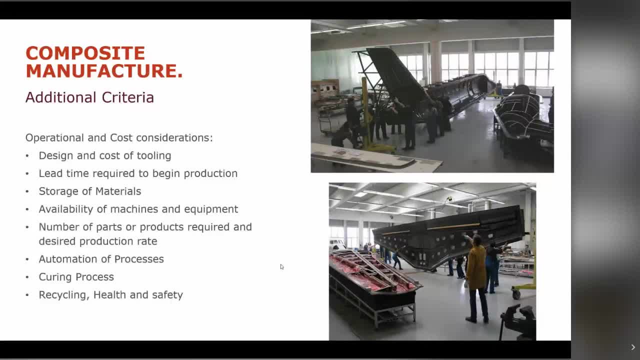 or get even material that might be supplied from a different place. Availability of machines and equipment: Machines and equipment are typically used for manufacturing of products, Therefore, that needs to be considered. I mentioned already that number of parts plays a significant role in selection. 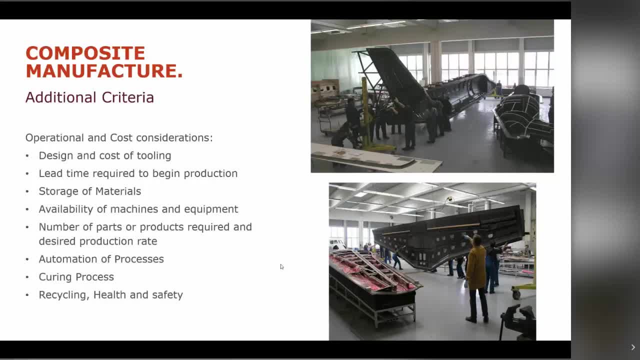 because, of course, that will give you ability to think about not only the process but also the tooling strategy and ability to recover the cost introduced. Same goes for the automation of the processes. However, what needs to be considered is the maturity of particular 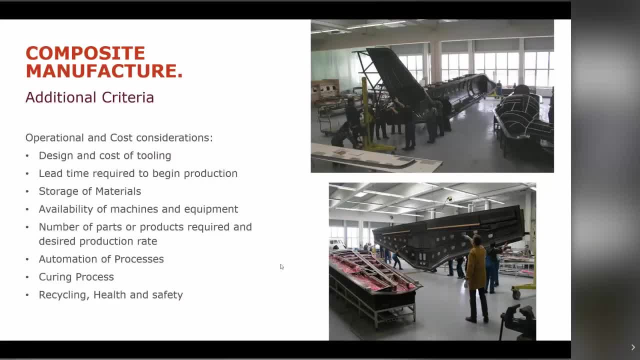 automation equipment for the given part of the process. In terms of curing processes, considerations such as is it autoclave, out of autoclave, do we have the capability and how to access it will need to be also considered Recycling and health and safety. 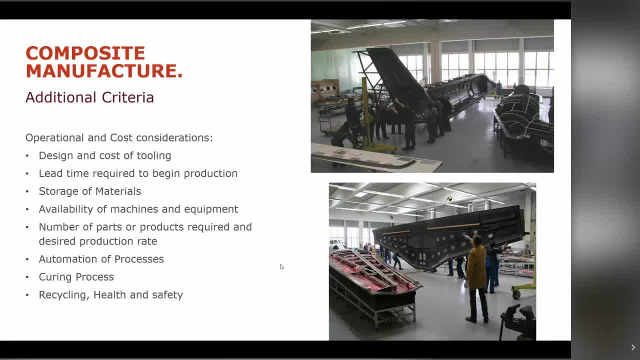 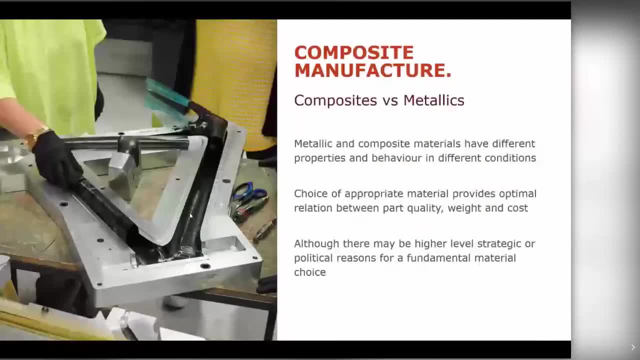 are absolutely critical. So when you manufacture composite parts, you're always thinking that must be because they're so significantly better than my counterparts. But composites are good for some things. however, they have their drawbacks too. They have slightly different properties and behaviours. 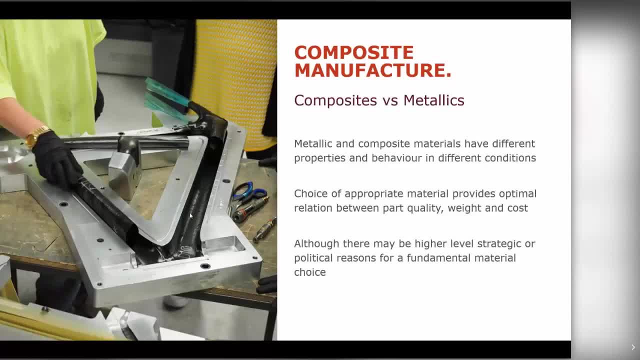 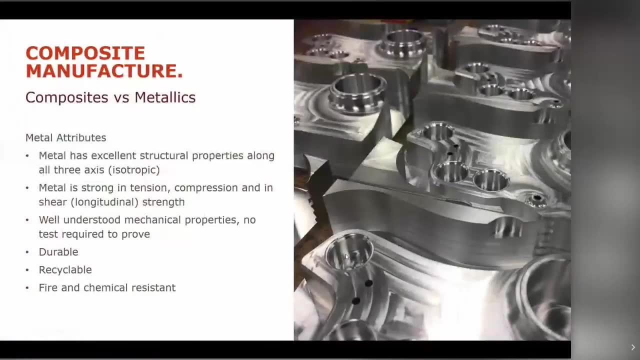 and one will need to be carefully considering those pros and cons, because composites, whilst they're good for particular applications, they might not be suitable for some. So, for example, metal has excellent structural properties along all three axes, which effectively makes designing. 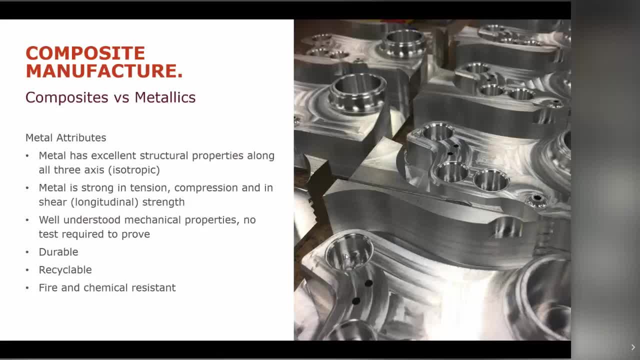 with metals relatively easy, So you don't need all those complex analytical tools to cater only for the complexity introduced by differing orientations. They're durable, recyclable, and we have been working with metals for quite a number of years. However, even though metals 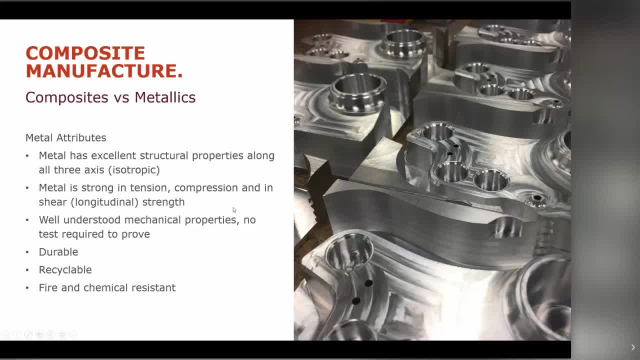 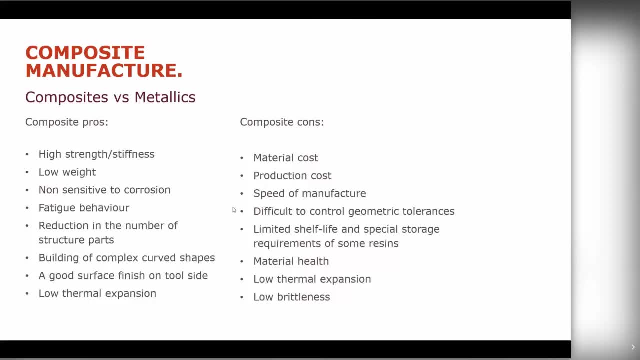 have those great characteristics. composites can and do fight back and they find their place and way into manufacture of high-value goods. They have high strength and stiffness, low weight, they could be designed to be non-sensitive to corrosion and they have a relatively good fatigue behaviour. 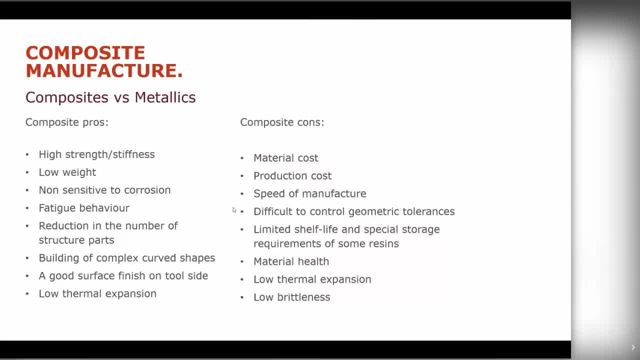 You can achieve reduction in number of parts, which in metallic counterparts is somewhat reduced, Building complex curve shapes achieving good surface finish, and they could get very low thermal expansion, especially with carbon fibre. On the negative side, the cost could be prohibitive, so one would need to 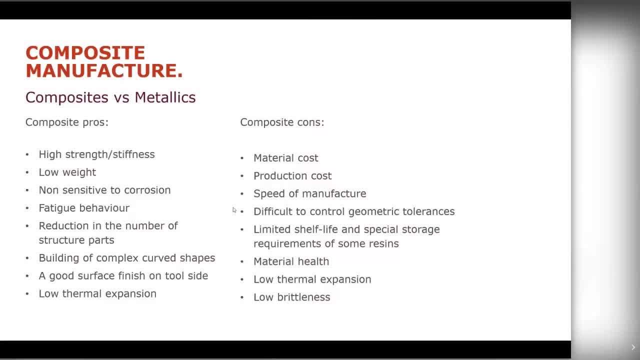 consider rather carefully the cost benefit and cost analysis in conjunction with design. That includes production cost, speed of manufacture. Sometimes it would be difficult to control geometric tolerances, and that is not purely dependent on the process, but also on the skill of your manufacturing workforce. so then, 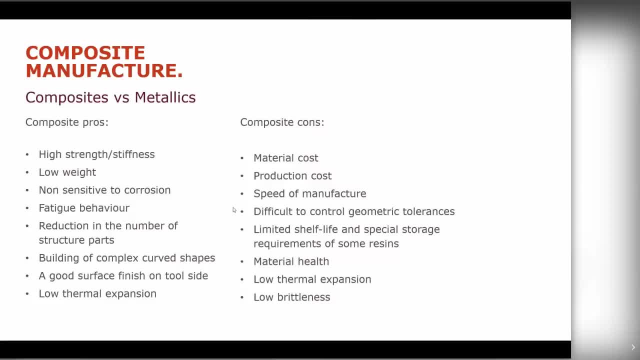 training requirement becomes quite significant. Some of the composite constituents have limited shelf life- The material health in that sense can be affected- and some of them have low brittleness, meaning that they can actually be rather easy to introduce damage. Okay, so I've tried in this webinar to 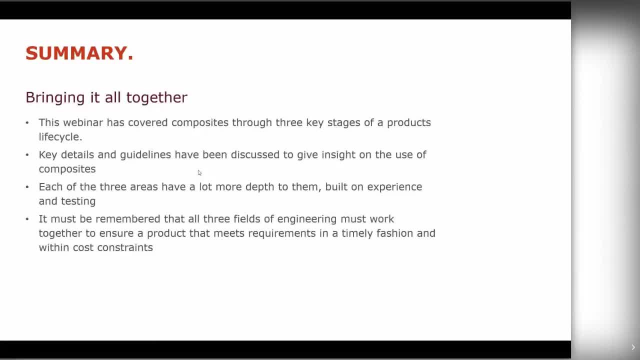 give you exposure to a variety of topics, considering composite, introduction, design, manufacture and some of the basic terminology that is needed to start the conversation. This is not the end of it. this is rather just the beginning, and I hope I managed to introduce the topic in a way that is interesting. 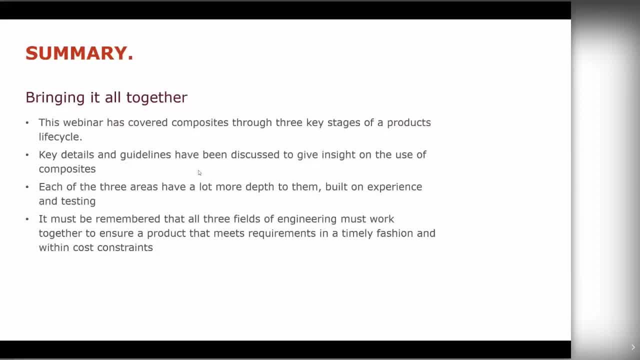 and might mean that you would want to pursue further interest in composites. We've divided the webinar into three key stages of the product life cycle, introduced the guidelines that help designers design the composites even before the heavy analytics starts, because they're very complex. those design guidelines. 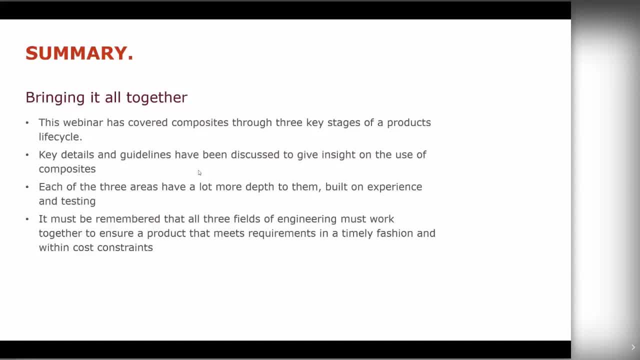 are absolutely necessary for designers to know how to start the initial concepts. As I mentioned, these areas have a lot more depth to them and there is more training needed effectively to understand the depth needed to design properly with those materials. Finally, I do want 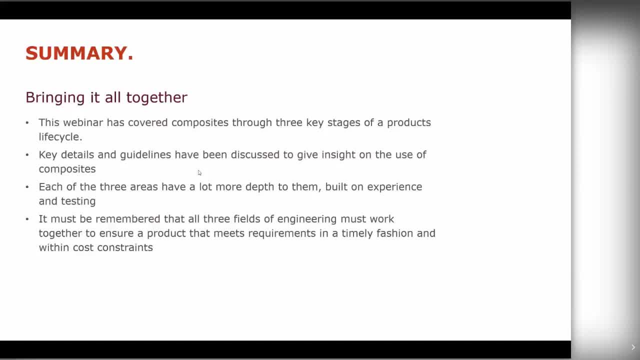 to stress one very important point that is built on my practical experience, and that is that, in order to deliver a good product, all different capabilities- ranging from engineering, design, stress, manufacturing, assembly, service and so on- need to work together in order to meet. 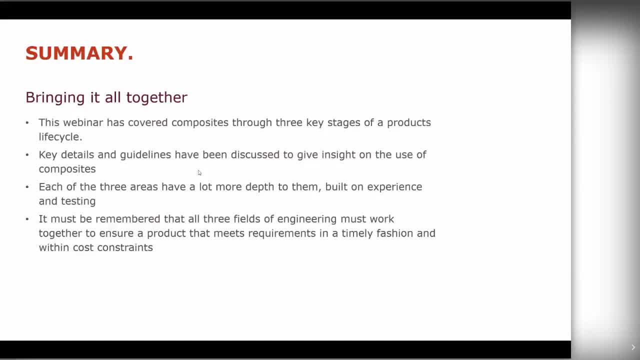 all the requirements and make the very useful product. The typical example of when they don't work together is that a product that is designed can simply not be manufactured, because it will not get out of the mold, for example. Very important to take out of this. 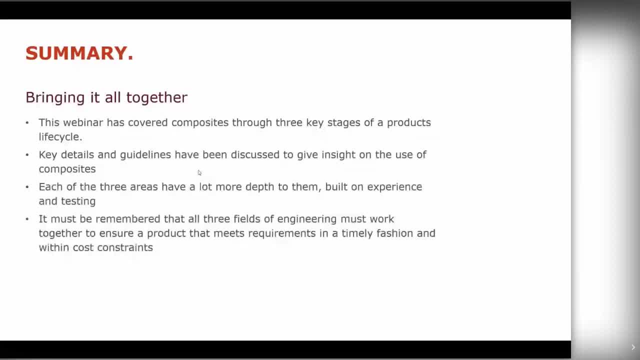 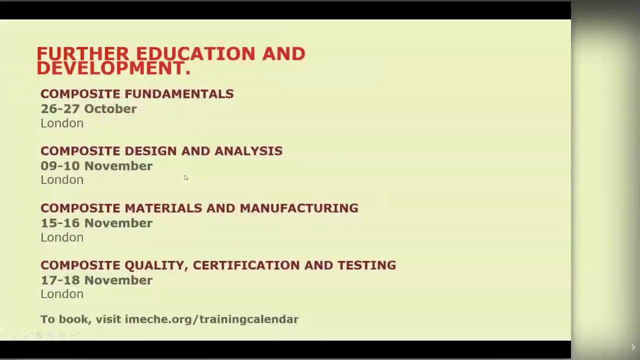 webinar is that all of the disciplines are absolutely interlinked and knowledge across the whole of the technology is necessary to deliver a good product. So that brings me to the end of this presentation and, as I mentioned, if there are any further interests, I Micky. 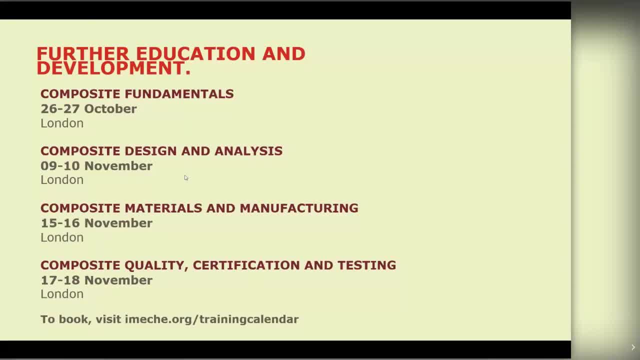 will be running some further trainings on the dates presented here. That's absolutely fantastic, Miroslav. Really appreciate your insight into all this and an introduction to this composite area. It's really fantastic. thank you so much for that. Actually, Miroslav, I have to say there's been 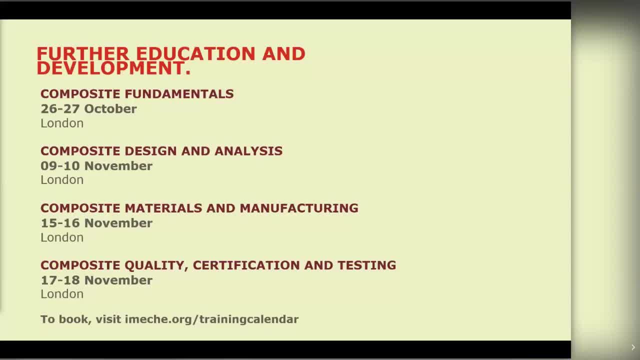 numerous questions coming in. There's been a lot of engagement on the chat box between individuals, which is great to see. Questions have been put out there and questions have been answered by other people that are on this webinar, which is great to see. I don't know if you've got. 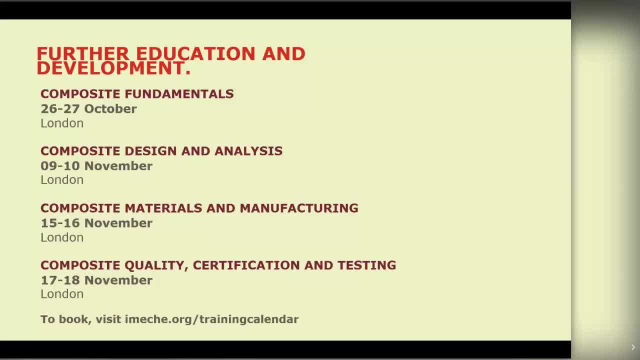 time to catch your breath. I'm conscious of time for everyone here because we've reached the hour, but I did promise we'd have some time for the Q&A. Are you okay to fire some questions at you, Miroslav? Absolutely, not a problem at all. 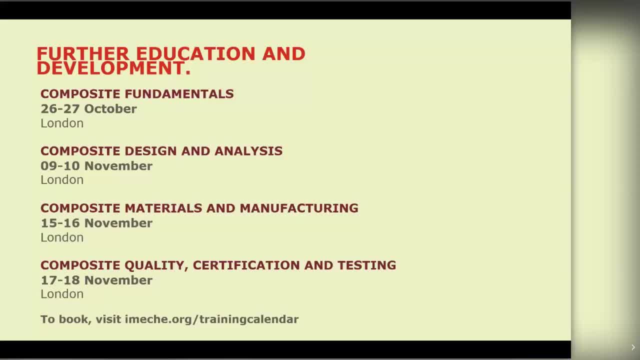 I'll keep straight with a very simple one, and actually a lot of people responded to this: How easy or viable is it to repair composites? The repair of composites is depending, really, first of all, on the sector we're talking about. If we are, for example, talking about 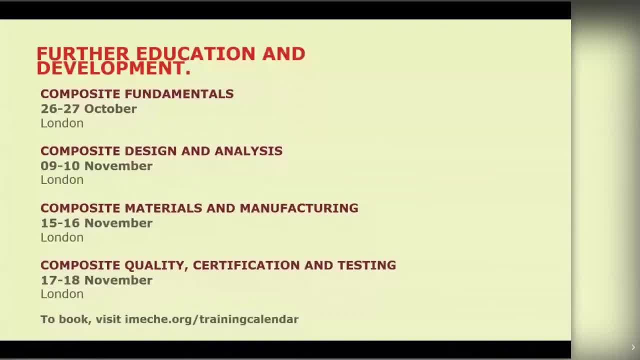 aerospace repair. that is a highly regulated area and one would need to consider them very early, almost during the design You would need to design for your repairs because of course, what you're repairing still need to maintain and hold the structural strength and performance as required. 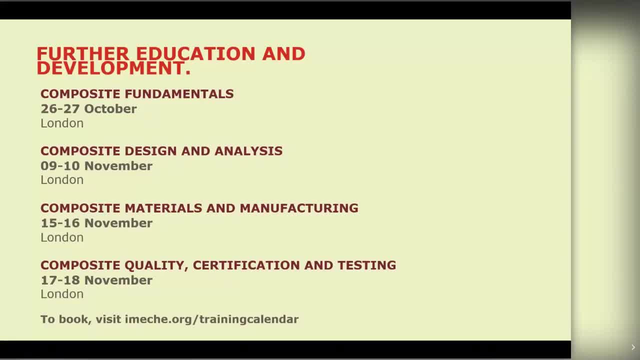 Some other areas of- I don't know- broad goods and where the structural requirement isn't that high are of course repairable, and it is a typical manufacturing procedure. One would need, of course, to consider: has the main structural component or main structural function of the part been? 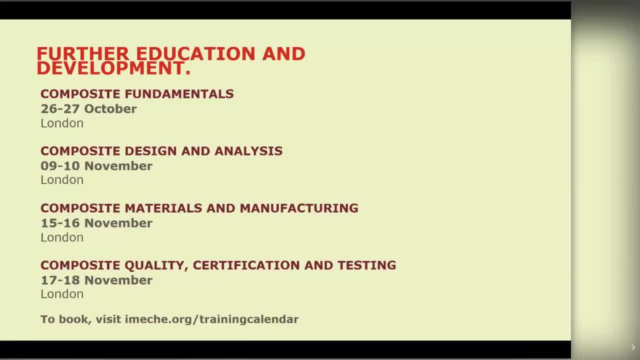 affected, and if so, probably some further design work would be needed, but absolutely it is possible. It is, however, highly advisable that, before you launch yourself into repairing composites, some assessment of what the component does- can it restore its original properties and features be achieved, and there would be. 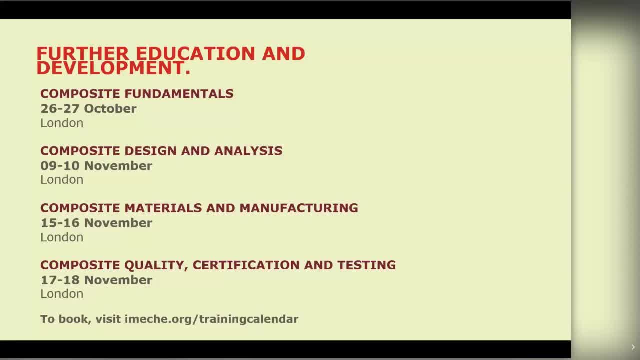 particular repair kits that you could use to do so, but it would be advisable that some assessment of the requirements is firstly made. Okay, fantastic, thank you, and just let you know there's some really good comments coming in from everybody thanking you for such a very informative. 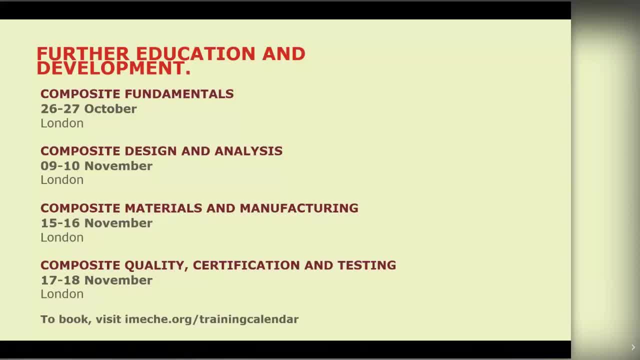 and good presentation, which is great. Another question here from Jonathan Harris: for you, what would be an indicative upper bound temperature for the use of composites in a load bearing application? Well, that's a very good question. if you're talking about matrix composites, let's say the. 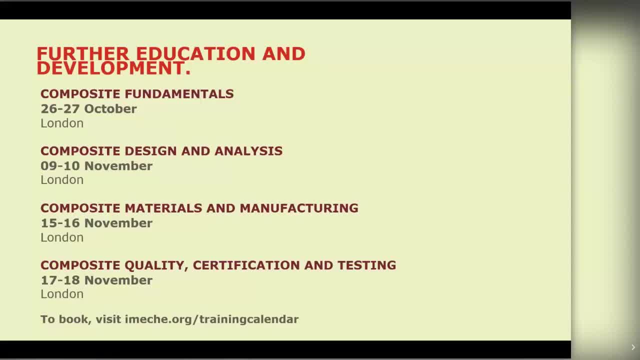 temperatures are typically the highest temperature would be probably catered with thermoplastic materials such as peak and peck going, I don't know. 350- 380 degrees is the melt temperature, so you probably want to go below this for your structural component in terms of epoxies. 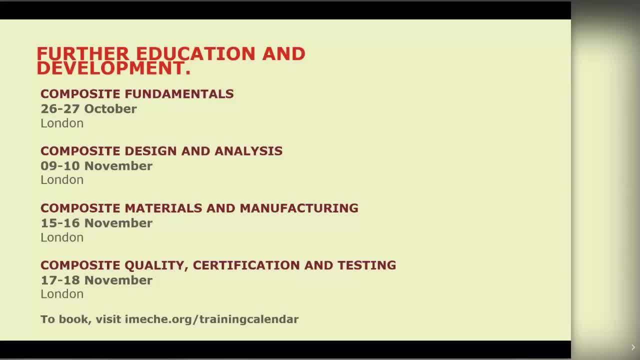 which are typically used in materials typically used in aerospace. yeah, depending on what epoxy resin you would use, the pure temperature is, I don't know, 180 degrees. so you probably you want to go not higher than 120-130 degrees at any point in time. really, 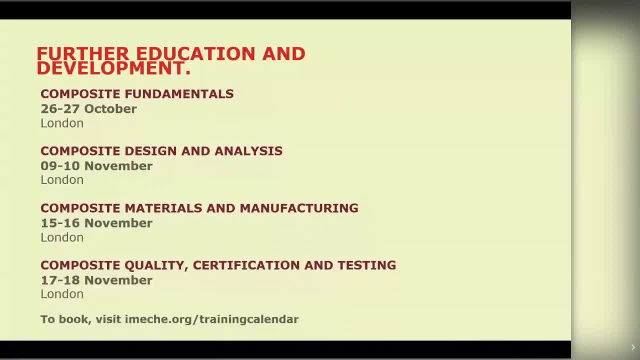 and even lower. so you really need to consider what material you want to use. if it is a really really really high temperature- extremely high temperature- organic matrix composites are probably not the right material choice for you. you probably want to look into ceramic matrices and stuff like that. 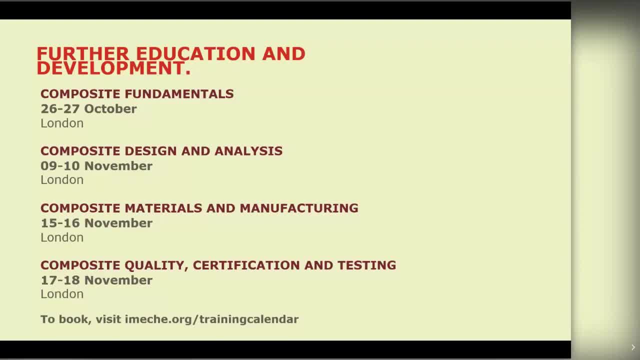 I was on mute. okay, thank you there. another question from John Hambly. he asked: if we move towards net zero, are composites a good choice and is there work going on to reduce their embodied carbon footprint? the simple answer is yes, there is works going on in this space. 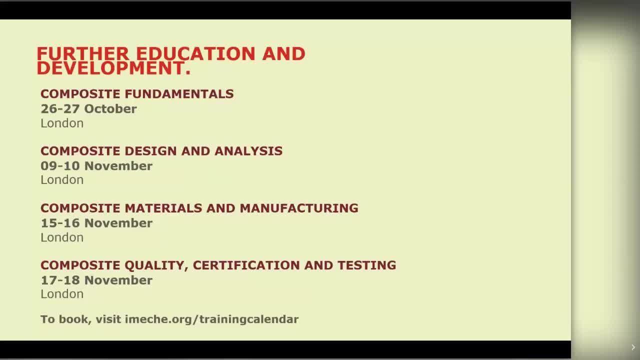 and we are all very conscious that recyclability is one of the things that composites are needing to meet in order to be environmentally friendly and, as suggested, at net zero. I do have to say that already, by the virtue of careful design, we are only really using. 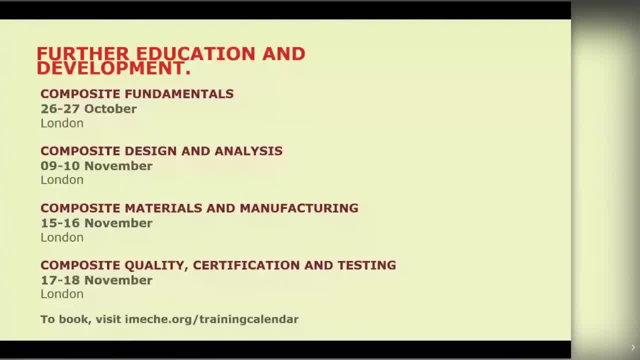 material as and when needed. so we are tailoring the material, and that reduces effectively waste and there are certainly automation efforts that enable higher yield of the raw material and less energy. but there is a lot more work needed to give you the full answer and I would say this is equally the 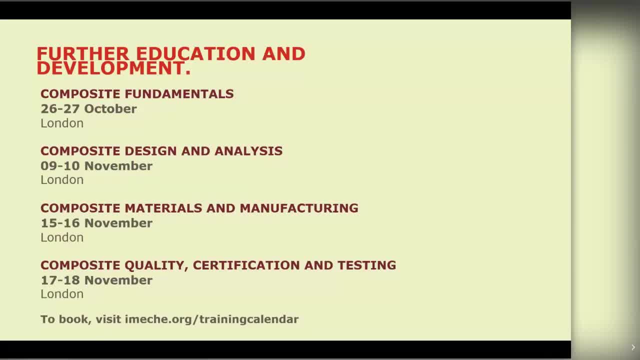 question for the rest of the manufacturing, as it is for composites. I think composites are making some good efforts to tackle this and there are projects- certainly that I know of- that are looking at this particular challenge. okay, fantastic, thank you again. this one is coming from. 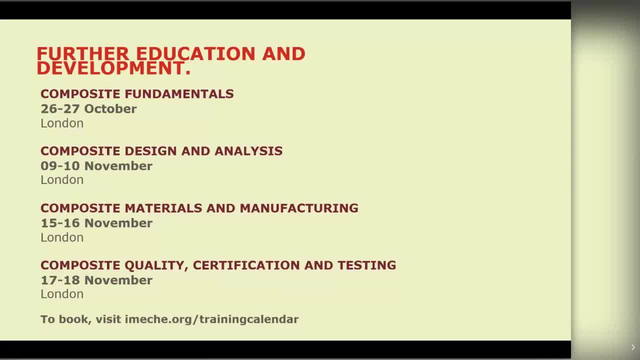 a bit of a longer question. how do you go about conducting tests to ensure the material had achieved its desired structural integrity or performance, and are there any considerations given to how the part performs in extremes of temperature or loads, etc. okay, well, it's a rather involved question, but 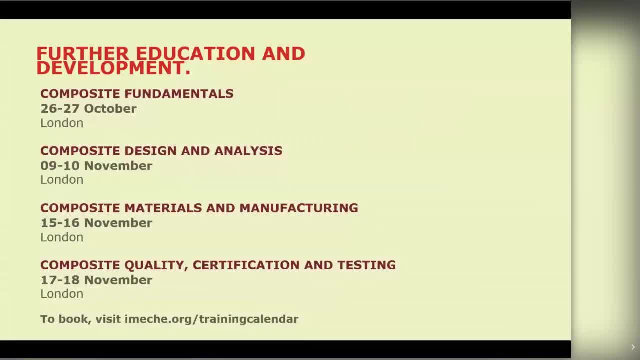 I'll try to answer. so testing is certainly one of the key things in making sure the composites are compliant with the design goal or requirement. I would always say- this is coming from me, from a very practical experience- if you are designing something and you have your, 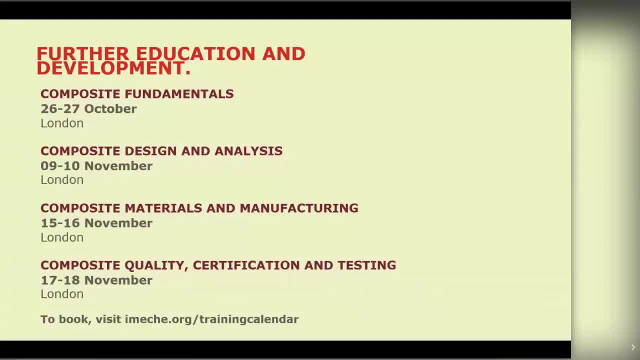 material properties based on some theoretical data. that's great. eventually, you would need to test and verify that your predictions are being met in reality. so how would you do so? you would need to consider a variety of test methods, and there is typically a typical approach in composites. 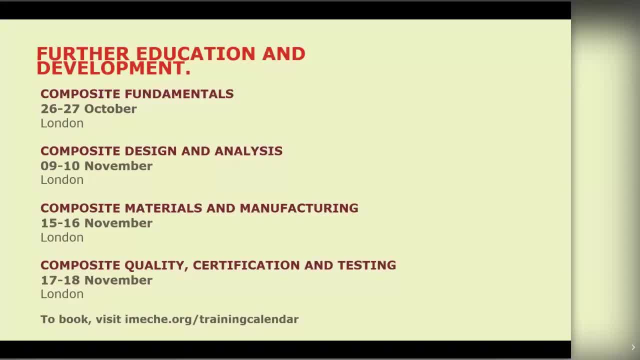 is running a pyramid of tests from the coupon level and going into feature level, sub assembly assembly and so on, increasing the complexity of the test and testing greater and greater components in the pyramid of tests. certainly the thermal exposure is one of the elements, but it's not the only one. it could be chemical. 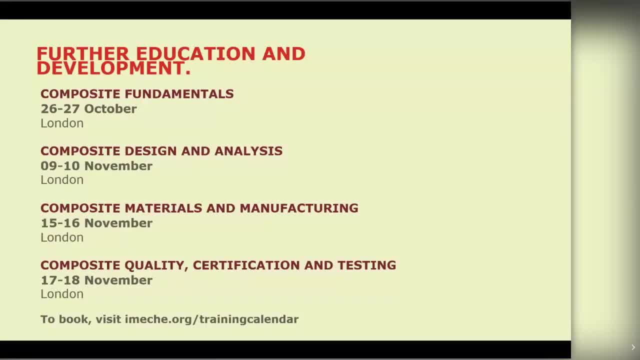 it could be UV exposure and so on. it really depends on what your component is trying to achieve. so it would be within your design goals or requirements what is required. so, for example, 25 year life in bright sunlight without UV degradation. so therefore, your test will certainly need to have an. 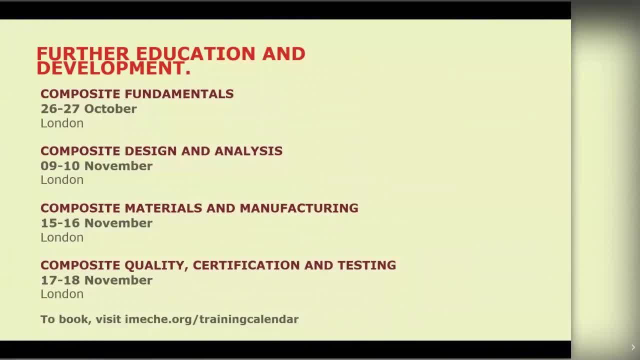 element that demonstrates that, and before you go into test- because these are very expensive- you'll probably need to do quite a lot of analysis, because you don't necessarily want your test to fail when you've invested so much into making a part brilliant, thank you. should we do one more question? 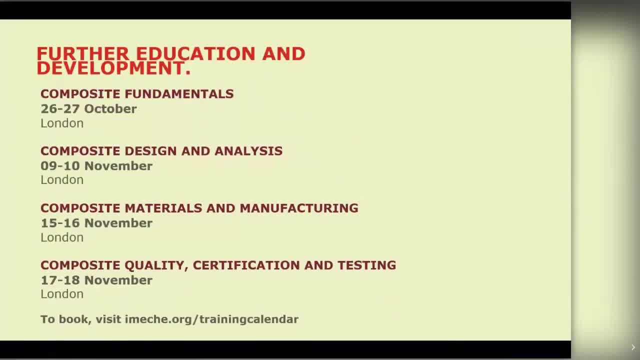 are you happy with that? yeah, it's fine. so this is from Daniel. for composites that do not have a laminate structure in brackets, MMCs or CMCs, or for think composites where laminate theory cannot be used, what is the analysis method using oriented 3D? 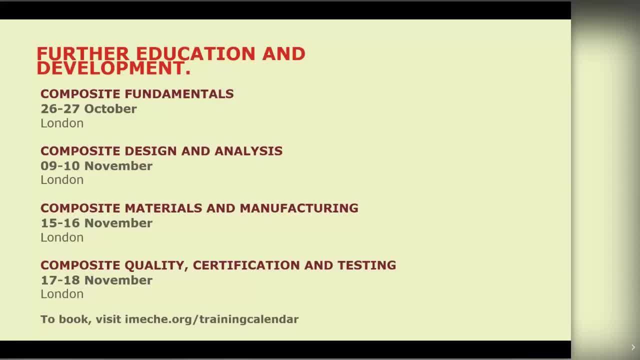 FE elements and 3D failure theories. right, okay, so if I understood the question, in this particular webinar we talked about laminated composites where the fiber is oriented across the particular direction, where that's unidirectional or perhaps woven. the question is about composites that have 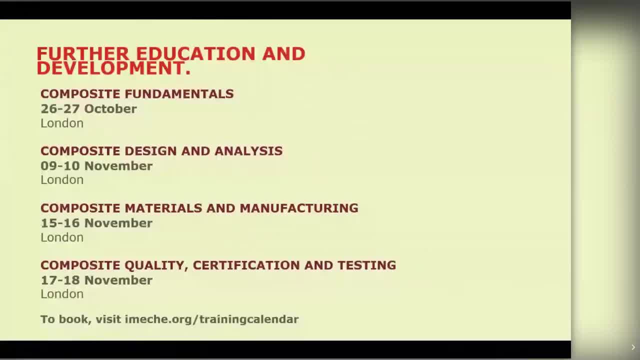 two constituents that are either particulates or some other forms within the combined with each other. so, for example, there is a variety of techniques that you could use. I'll give you one that I have used and know of. there are particular tools that could model the, let's say, unit. 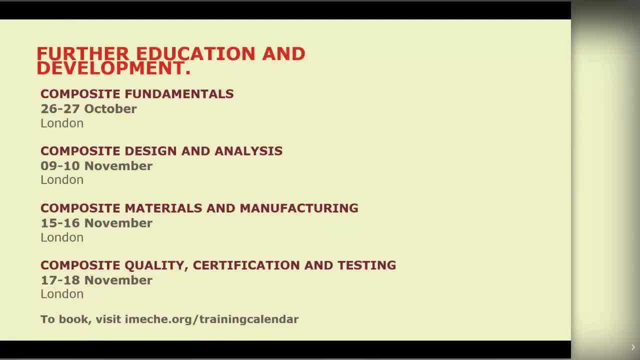 cell of your material where you would actually model, the reinforcing material being your particulate and also your matrix being enveloping material. so if you're talking about metal, matrix composites would be your- I don't know metal that envelopes the particle that is within it, or 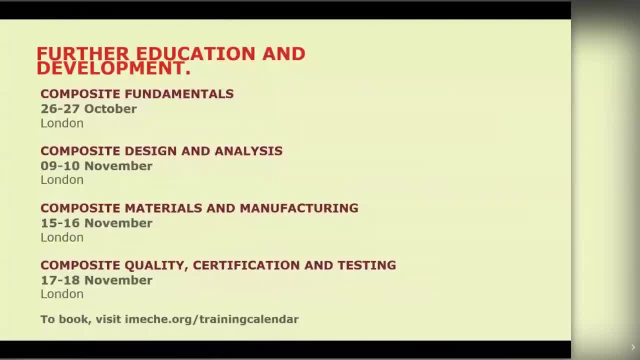 number of, and you would need to model it at a micro scale to get your response. that response is your effective material model that you can use in designing the overall part. of course, this is a very simplified methodology because it will give you just the first strength and stiffness.